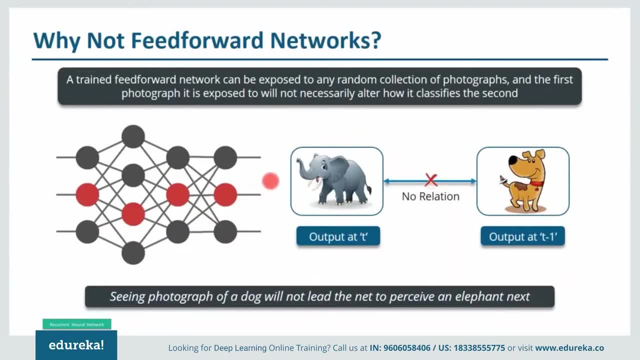 a relevant label to that particular image as well. Now, if you notice, the new output that we have got that is classifying an elephant has no relation with the previous output that is of a dog. Or you can say that the output at time t is independent of. 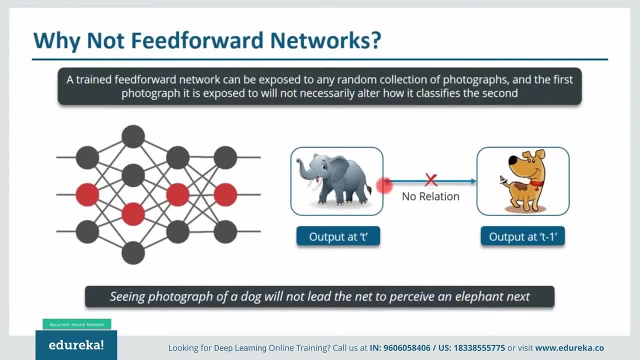 output at time t minus one, As we can see that there is no relation between the new output and the previous output. So we can say that in feedforward networks outputs are independent to each other. Now there are few scenarios where we actually need the previous output to get the new output. Let us discuss. 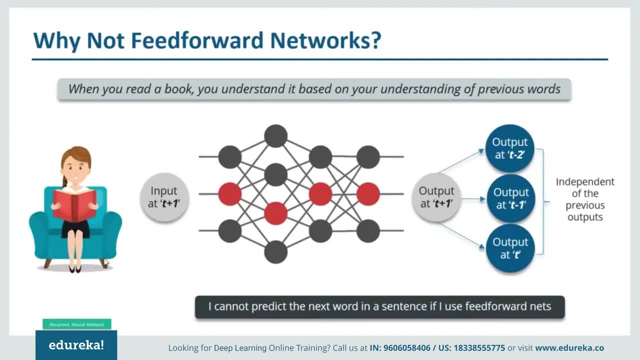 one such scenario. Now, what happens when you read a book? You'll understand that book only on the understanding of your previous words. Alright, so if I use a feedforward network and try to predict the next word in a sentence, I can't do that. Why can't I do that? Because 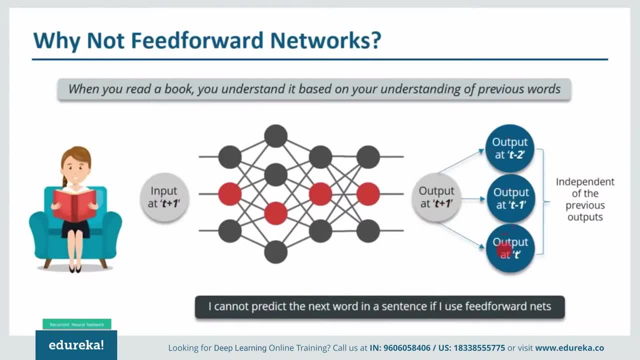 my output will actually depend on the previous output, On the previous outputs, But in the feedforward network my new output is independent of the previous outputs. that is, output at t plus one has no relation with output at t minus two, t minus one and at t. So basically we cannot use feedforward networks for predicting. 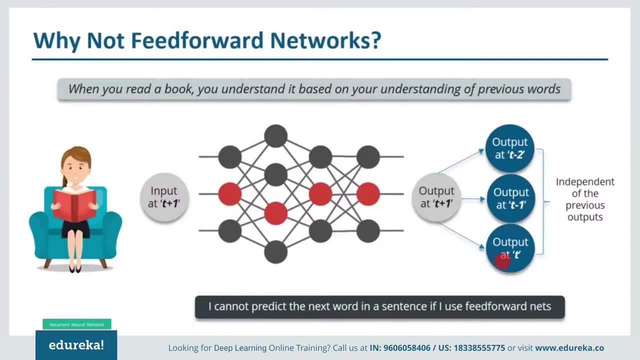 the next word in a sentence. Similarly, you can think of many other examples where we need the previous output, some information from the previous output, so as to infer the new output. This is just one small example. there are many other examples that you can. 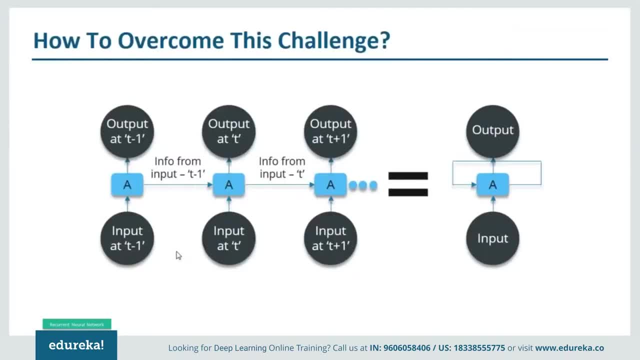 think of. So we'll move forward and understand how we solve this particular problem. So over here what we have done: we have input at t minus one, we'll feed it to our network. then we'll get the output at t minus one. Then at the 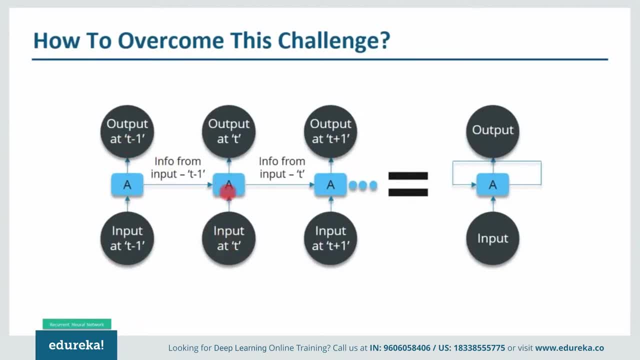 next timestamp, that is, at time t, we have input at time t that'll be given to our network along with the information from the previous timestamp, that is, t minus one, And that will help us to get the output at t. Similarly, at output for t plus one, we have two inputs. 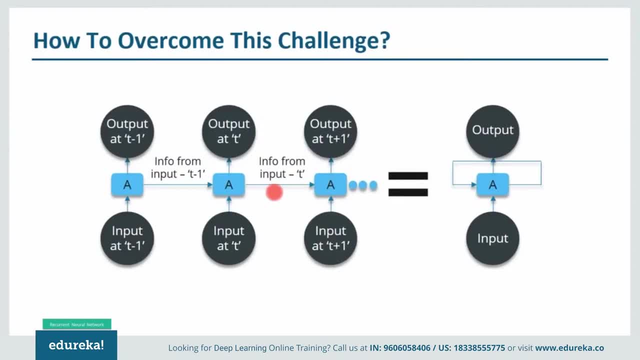 One is a new input that we give. Another is the information coming from the previous time timestamp, that is t, in order to get the output at time. t plus one. Similarly, it can go on So over here. I have just written a generalized way to represent it. There's a. 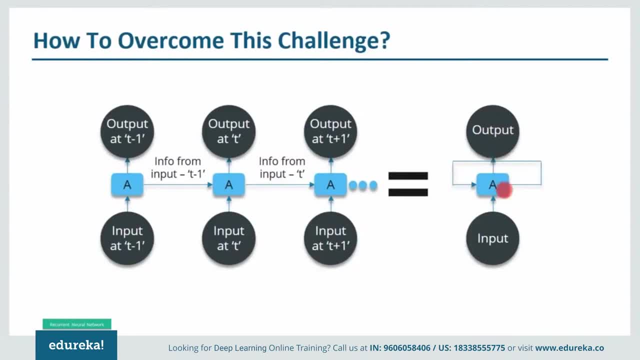 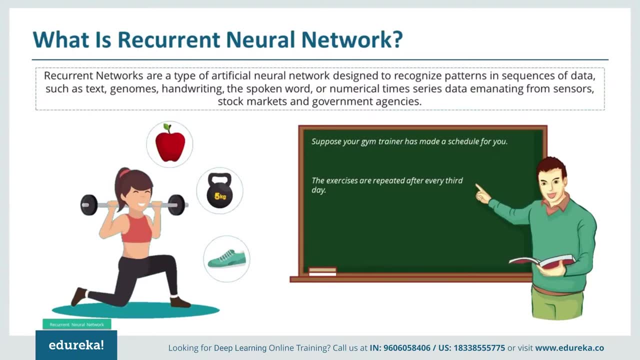 loop where the information from the previous timestamp is flowing, and this is how we can solve this particular challenge. Now let us understand what exactly are recurrent neural networks. So for understanding recurrent neural network, I'll take an analogy. Suppose your gym trainer has made a schedule for you. The exercises are repeated after every third day. 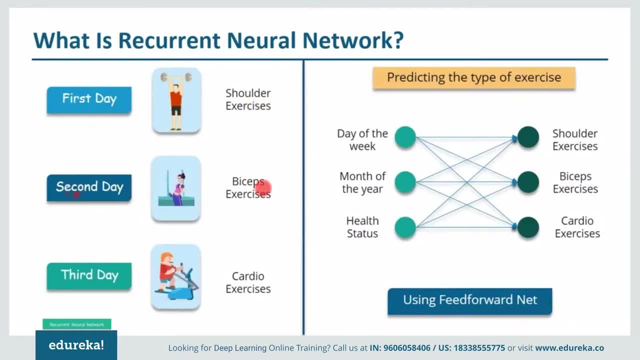 Now this is the order of your exercises. For example, if you're doing a workout, you're going to be doing shoulder. second day, you'll be doing biceps. third day, you'll be doing cardio, And all these exercises are repeated in a proper order. Now what happens when we 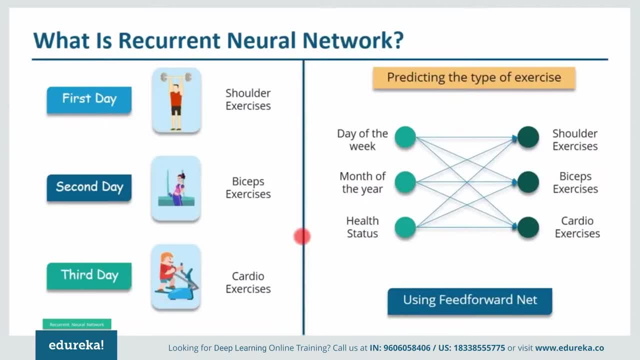 use a feedforward network for predicting the exercise today. So we'll provide in the input, such as day of the week, month of the year and health status. All right, and we need to train our model or our network on the exercises that we have done in the past. After that, 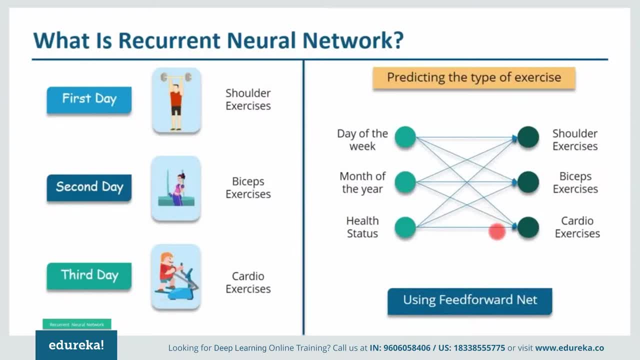 there'll be a complex voting procedure involved that will predict the exercise for us, And that procedure won't be that accurate. So whatever output we'll get won't be accurate as accurate as we want it to be. Now, what if I change my inputs and I make my inputs? 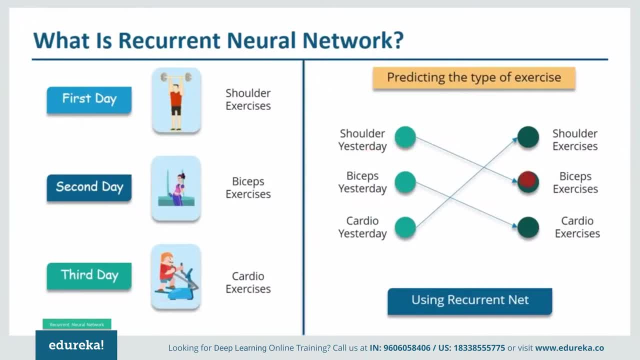 as what exercise I've done yesterday. So if I've done shoulder, then definitely today I'll be doing biceps. Similarly, if I've done biceps yesterday, today I'll be doing cardio. Similarly, if I've done cardio yesterday, today I'll be doing shoulder. Now there can. 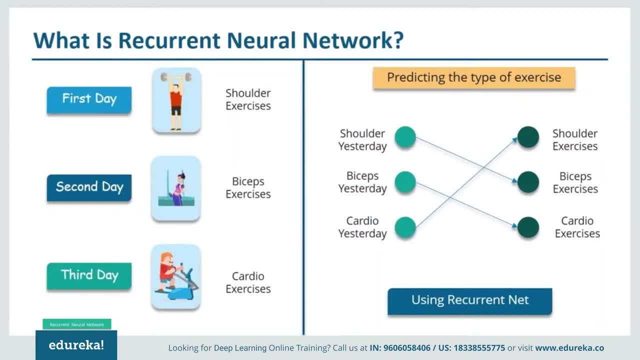 be one scenario where you are unable to go to gym for one day Due to some personal reasons. you could not go to the gym. Now what'll happen at that time? We'll go one time stamp back at yesteraday. So if the exercise that happened the day before yesterday was shoulder, then 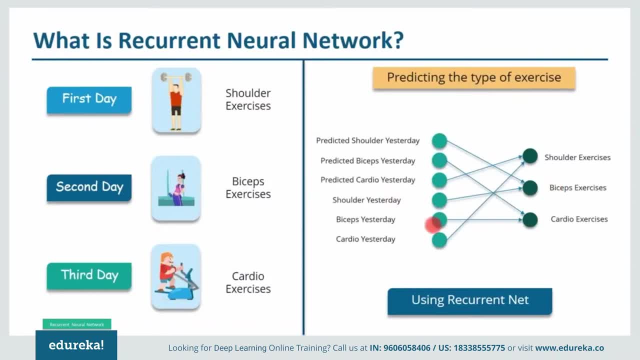 yesterday there are biceps exercises, Alright. Similarly, biceps happen day before yesterday, then yesterday would have been cardio exercises. Similarly, if cardio would have happened day before yesterday, yesterday would have been shoulder exercises. Alright. And this prediction, the prediction for the exercise that happened yesterday, will be fed back to our network. 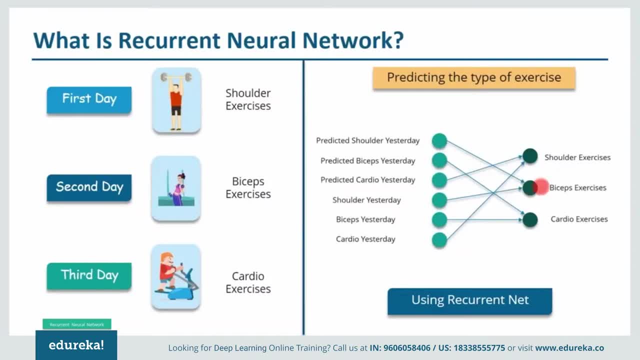 and these predictions will be used as inputs in order to predict what exercise will happen today. Similarly, if you have missed your gym, say, for two days-, three days or one week, so you need to roll back, you need to go to the last day when you went to. 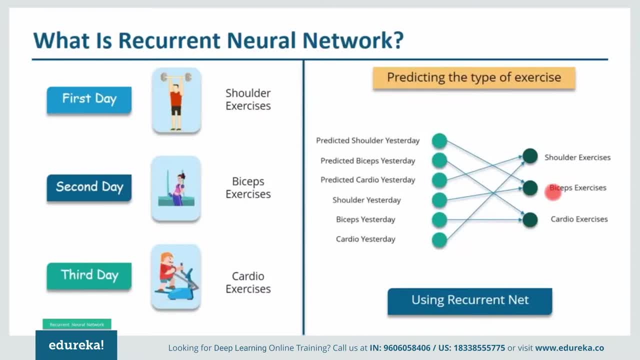 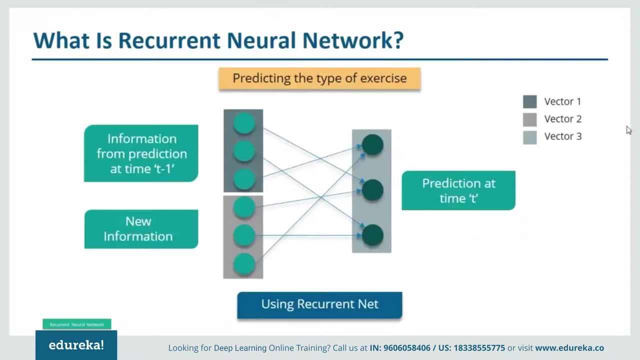 the gym. you need to figure out what exercise you did on that day, feed that as an input, and then only you'll be getting the relevant output as to what exercise will happen today. now what i'll do? i'll convert these things into a vector. now, what is a vector? vector is nothing but a list of numbers. 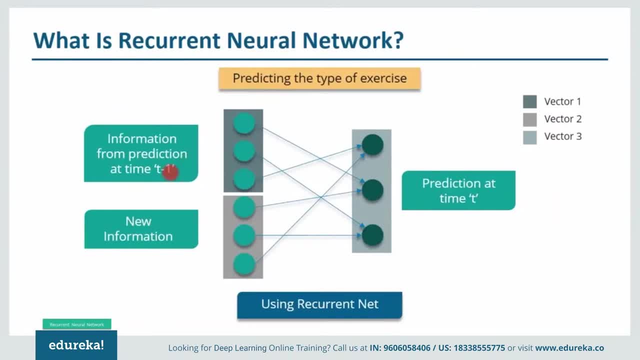 all right. so this is a new information, guys, along with the information from the prediction at the previous time step. so we need both of these in order to get the prediction at time. t imagine if i have done shoulder exercises yesterday, so this will be one. this will be zero. this will be. 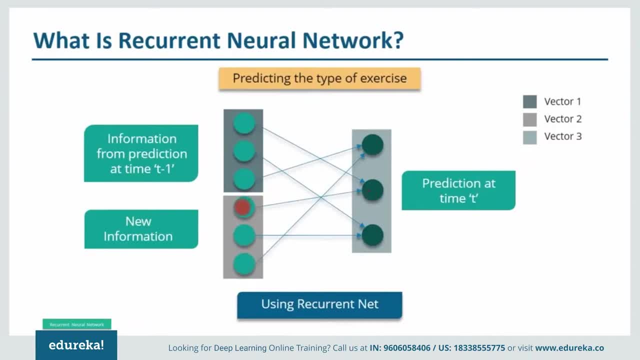 zero. now the prediction that will happen will be biceps exercise, because if i've done shoulder yesterday, it will be biceps, so my output will be zero. one and zero. and this is how vectors work, guys. so i hope you have understood this, guys. now this is how our neural network looks like, guys. 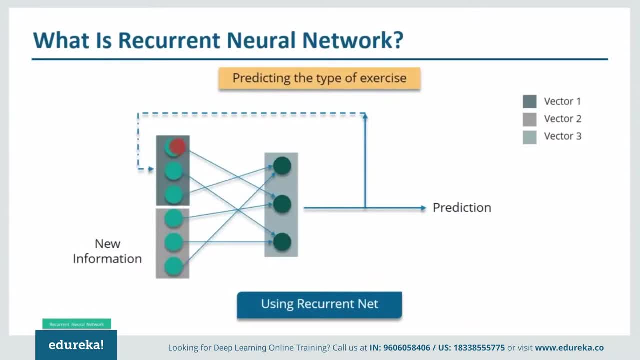 we have new information along with the information from the previous time stamp. the output that we have got in the previous time stamp will use certain information from that will feed into our network as inputs and then that will help us to get the new output. Similarly, this new output that we have got will take some information from that. 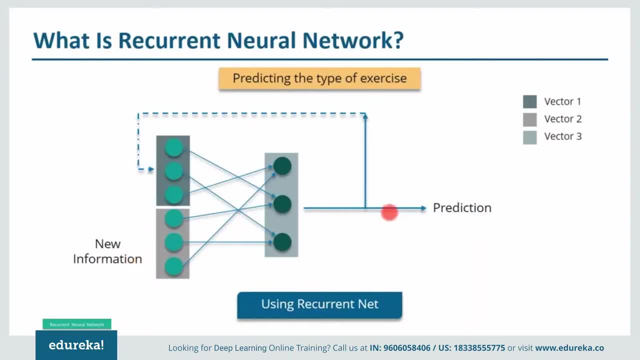 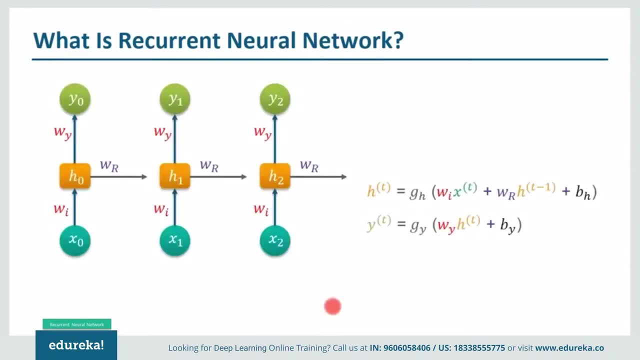 feed in as an input to our network, along with the new information, to get the new prediction, and this process keeps on repeating. Now let me show you the math behind the recurrent neural networks. So this is the structure of a recurrent neural network, guys. 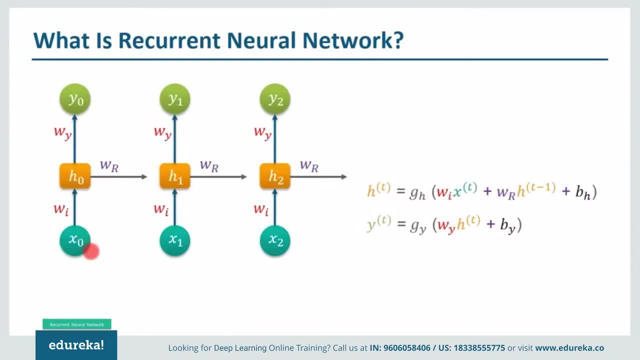 Let me explain you what happens here. Now consider a time. t equals to 0, we have input x naught and we need to figure out what is h naught. So according to this equation, h of 0 is equal to wi weight matrix multiplied by our input x of 0. 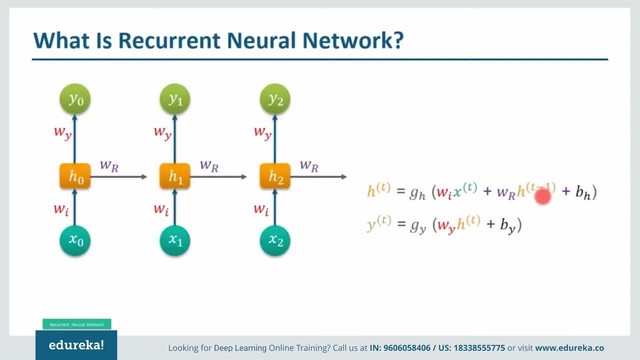 plus wr into h of 0 minus 1, which is h of minus 1, and time can never be negative, So with this particular equation cannot be applied here plus a bias. So wi into x of 0 plus bh passes through a function g of h to get h of 0 over here. 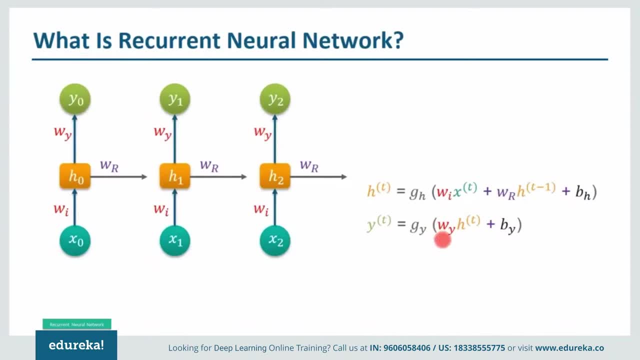 After that I want to calculate y naught. So for y naught I will multiply h of 0 with the weight matrix wi and I'll add a bias to it and pass it through a function g of y to get y naught. 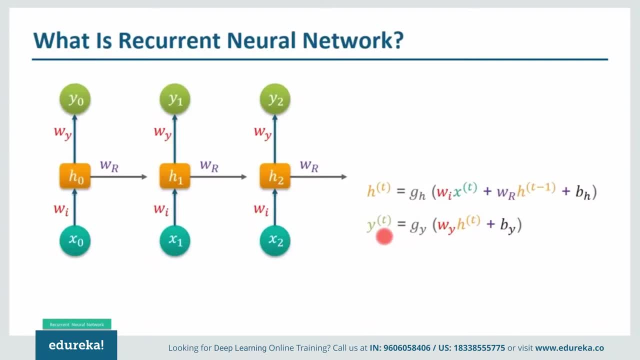 Now, in the next time stamp, that is, at time t equals to 1, things become a bit tricky. Now let me explain you what happens here. So at time t equals to 1, I have input x 1. I need to figure out what is h 1.. 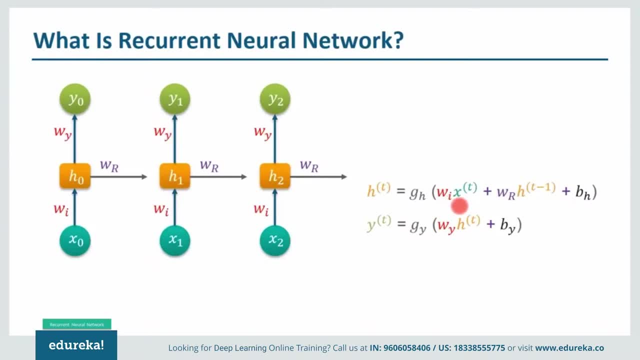 So for that I'll use this equation. So I'll multiply wi, that is a weight matrix, by the input x, 1 plus wr, into h of 1 minus 1, which is 0, h of 0.. We know what we got from here. 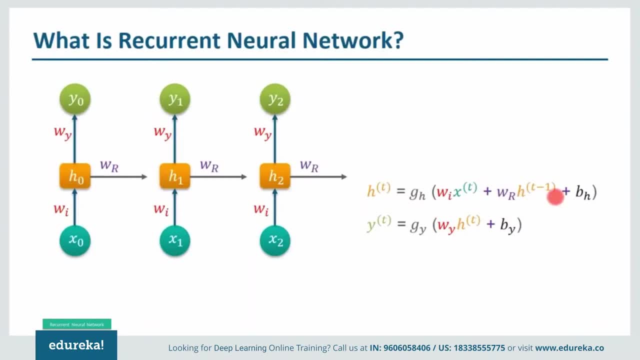 So wr into h of 0 plus the bias, pass it through a function g of h to get the output as h 1.. Now this h 1 we'll use to get y 1.. We'll multiply h 1 with wi plus a bias and we'll pass it through a function g of y to get y 1.. 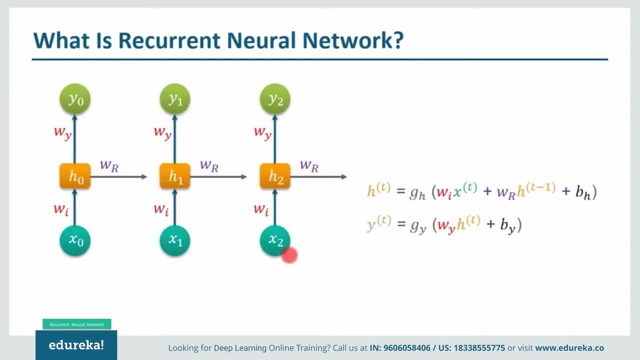 Similarly, the next time stamp, that is at time t equals to 2, we have input x 2.. We need to figure out what will be h 2.. So we'll multiply the weight matrix wi with x of 2 plus wr into h of 1 that we have caught here, plus b of h, and pass it through a function g of y. 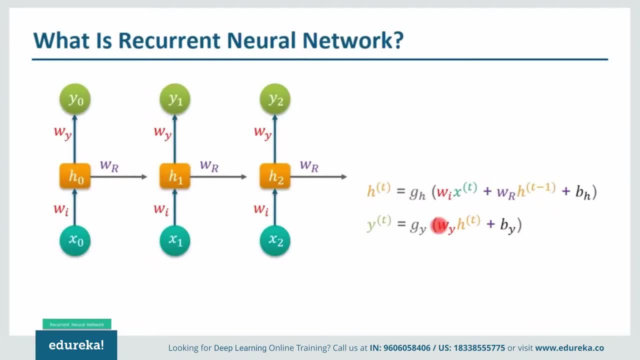 a function g of h to get h of 2. from h of 2 will calculate y of 2 wy into h of 2 plus by. that is the bias. pass it through a function g of y to get y. and this is how recurrent neural network works. 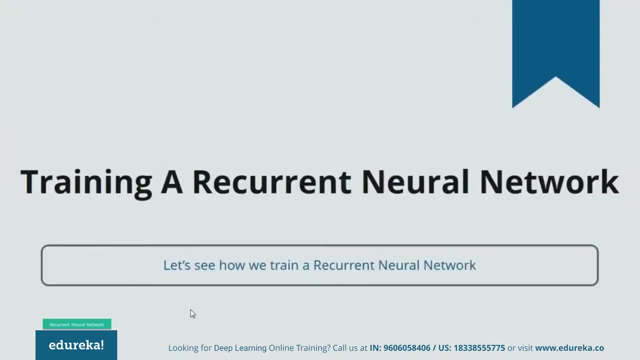 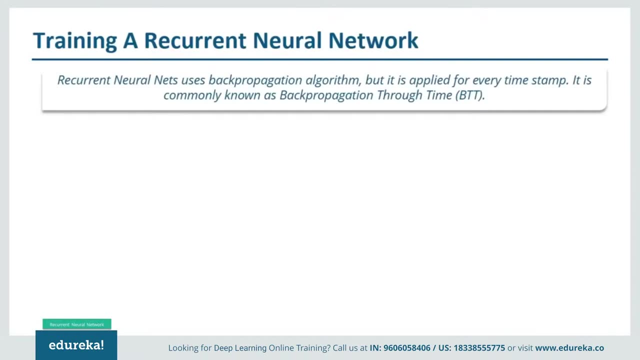 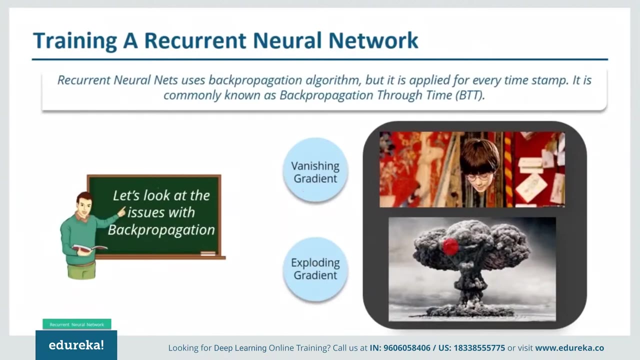 guys, now you must be thinking how to train a recurrent neural network. so a recurrent neural network uses back propagation algorithm for training, but back propagation happens for every time stamp. that is why it is commonly called as back propagation through type. now, with back propagation, there are certain issues, namely vanishing and exploding gradients. let us see. 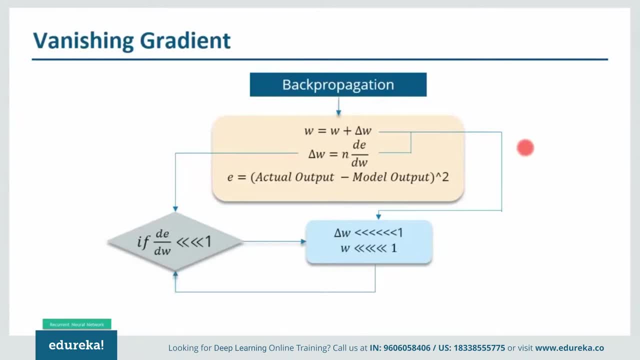 those one by one. so in vanishing gradient, what happens when you use back propagation? you tend to calculate the error, which is nothing but the actual output that you already know, minus the model output, output that you got through your model- and the square of that. so you figure out. 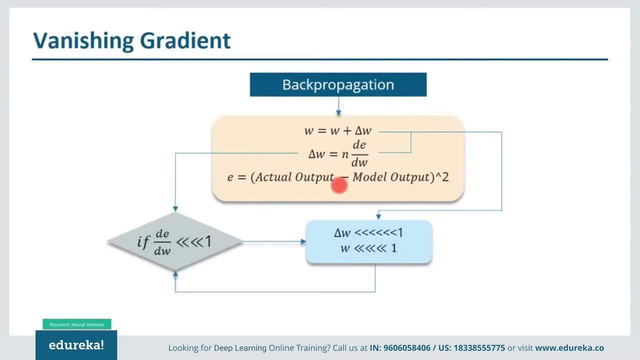 the error. with that error, what do you do? you tend to find out the change in error with respect to change in weight or any variable, so we'll call it weight here. so the change of error with respect to weight multiplied by learning rate will give you the. 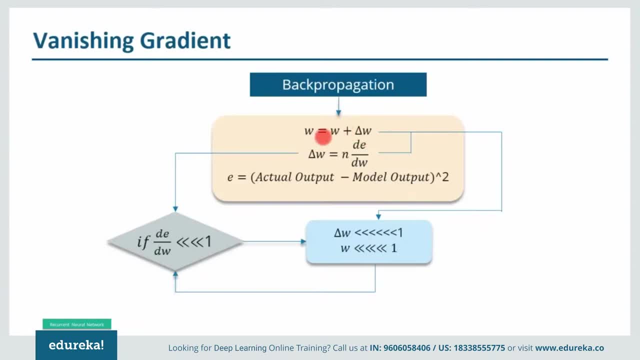 change in weight, then you need to add that change in weight to the old weight to get the new weight all right. so obviously what we are trying to do, we are trying to reduce the error. so for that we need to figure out what will be the change in error if my variables are changed right, so that 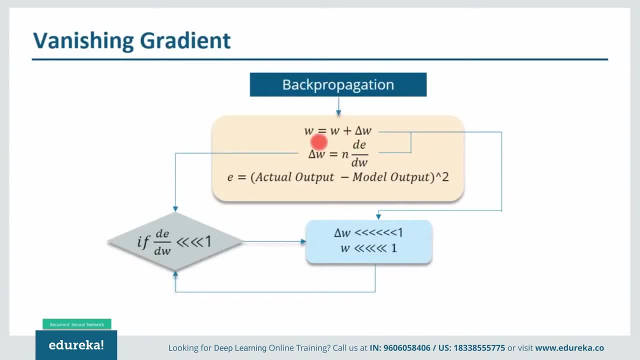 way we can get the change in the variable and add it to our old variable to get the new variable now over here. what can happen if the value d e by d w, that is a gradient or you can say the rate of change of error anymore in the variable- it is a very small error with respect to our variable. weight becomes very. 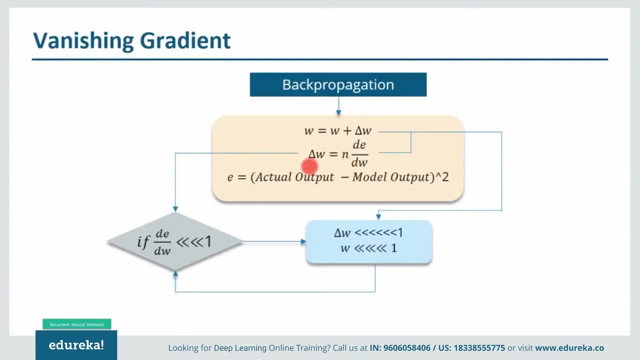 small than one, like it is point zero, zero, something. so if you multiply that with the learning rate, which is definitely smaller than one, then you get the change of weight which is negligible. all right, so there might be certain examples where you know you are trying to predict. say our next word in a 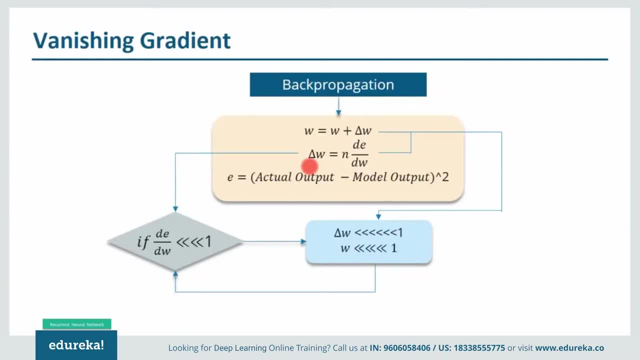 sentence and that sentence pretty long. for example, if I say: I went to France, dash, dash, dash, I went to now I need to predict speak what will come after speak. so for that I need to go back in time and check what was the context, which will be very complex, and due to that, there will be a lot of 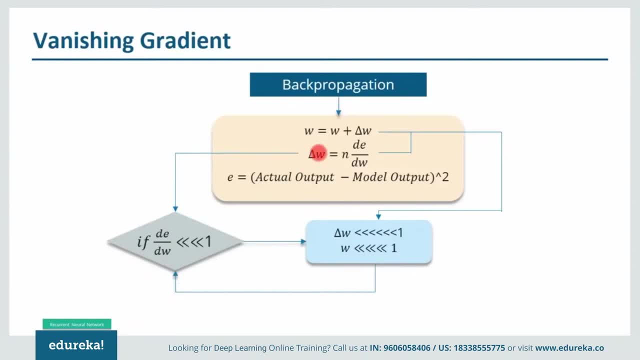 iterations and because of that, this error, this change in weight will become very small, very small. so the new weight that we'll get will be actually almost equal to your old weight. so there won't be any updation of weight. that will be happening, and that is nothing but your vanishing. 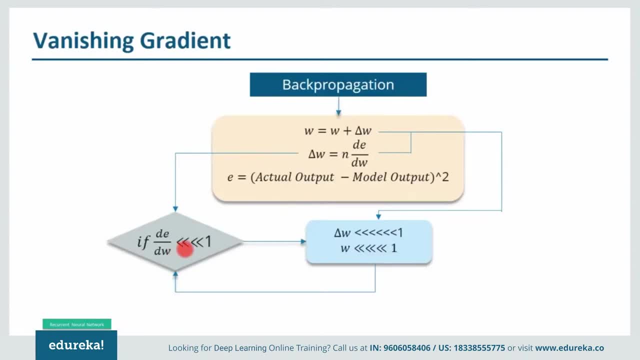 gradient. all right, I'll repeat it once more. so what happens in back propagation? you first calculate the error. this error is nothing but the difference between the actual output of the model output and the square of that. with that error we figure out what will be the change in. 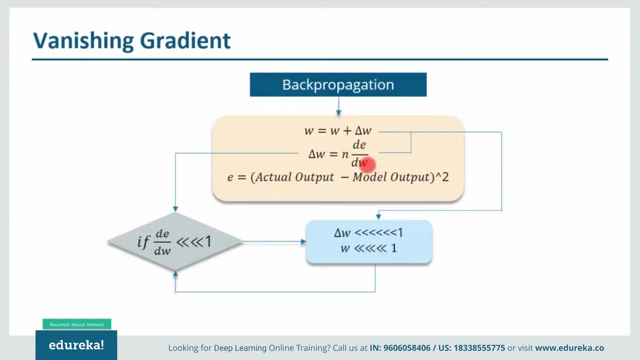 error when we change a particular variable, say weight. so d e by d w, multiplied with learning rate to get the change in the variable or change in the weight. now we'll add that change in the weight to our old weight to get the new weight. this is what back propagation is, guys. all right. 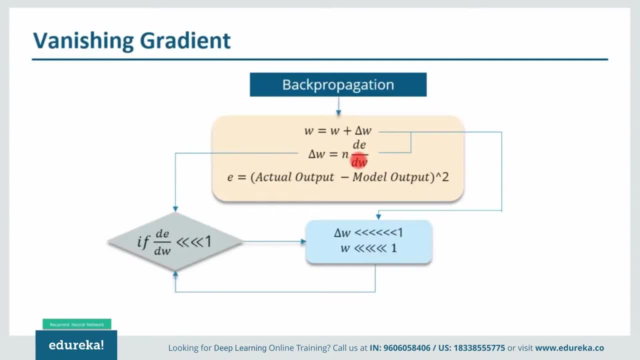 I'm just giving you a small introduction to back propagation. now consider a scenario where you need to predict the next word in the sentence and your sentence is something like this: I have been to France. then there are a lot of words, after that, few people speak, and then you need to predict what comes after: speak now. if I need to do that, I need to. 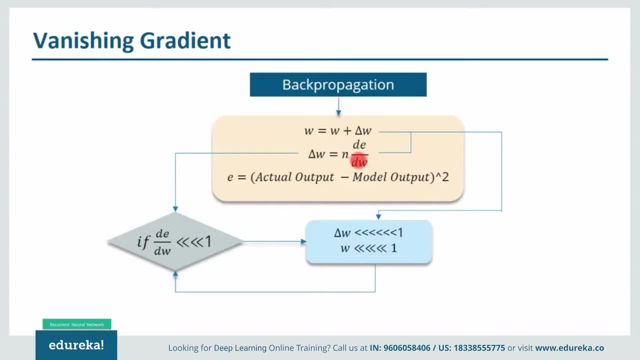 go back and understand the context. what is it talking about? and that is nothing but your long term dependencies. so what happens during long term dependencies? if this d e by d w becomes very small, then when you multiply it with n, which is again smaller than one, you get delta w, which will be very, very small. that will be. 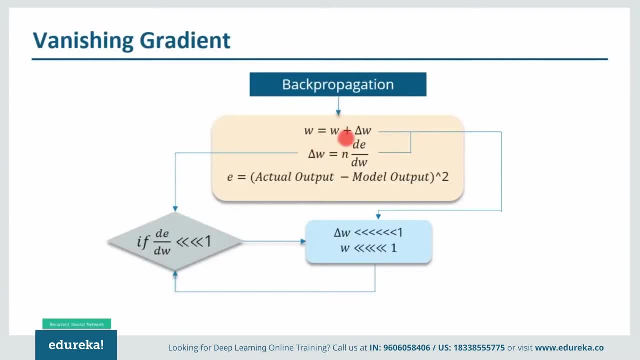 negligible. so the new weight that you'll get here will be almost equal to your old weight. so I hope you're getting my point. so this new weight- so there will be no updation of weights, guys- this new weight will definitely be, will always be almost equal to our old weight. there won't be. 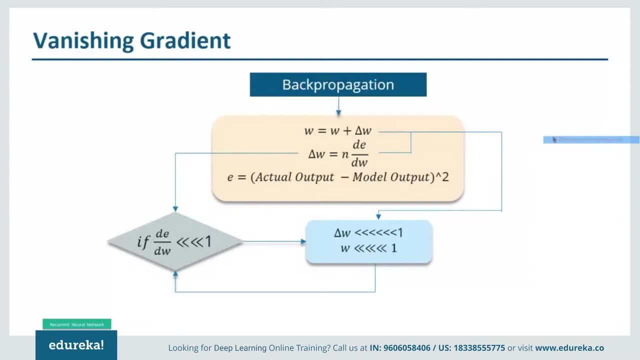 any learning here. so that is nothing but your vanishing gradient problem. similarly, when I talk about the gradient thing, what I call a gradient, you can say I bring here delta, w in this very long term dependencies. and so what happens when your gradient, or d e by d w, becomes very large? 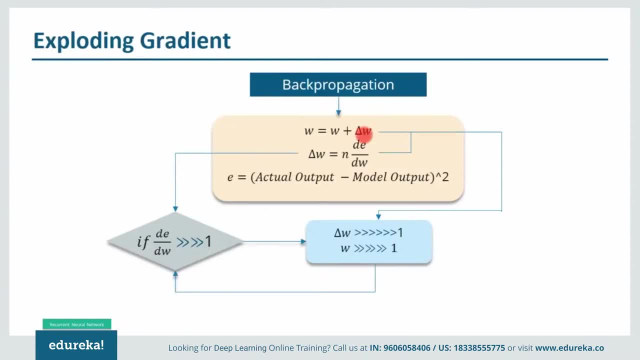 becomes greater than greater than one, all right, and you have some long term dependencies. so at that time your d by d w will keep on increasing. delta w will become large and because of that your weights- then you weight with that will come- will be very different from your old weight. so 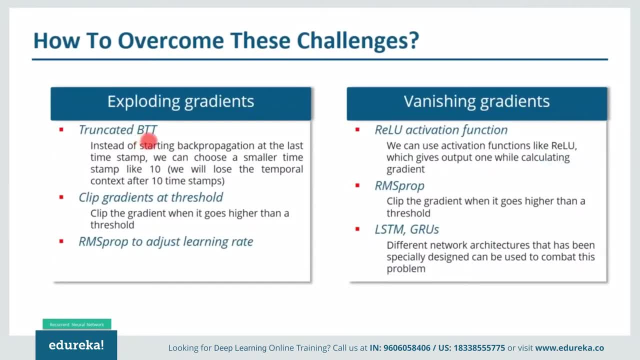 these two are the problems with back propagation. now let us see how to solve these problems now, starting back propagation. at the last time stamp. we can choose a smaller time stamp, like 10.. Or we can clip the gradients at a threshold, So there can be a threshold value where we can. 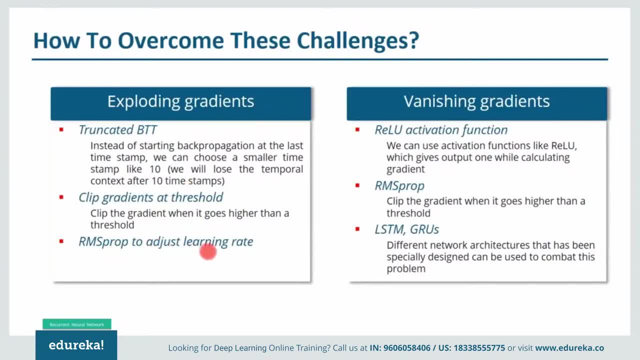 you know, clip the gradients And we can adjust the learning rate as well. Now for vanishing gradient, we can use a ReLU activation function. We have discussed ReLU activation function in artificial neural network tutorial guys. Similarly, we can also use LSTM and GRUs. 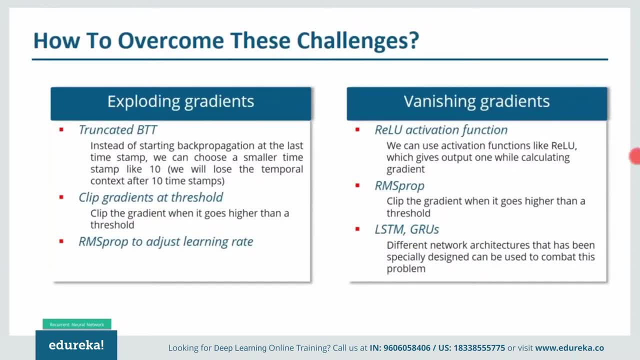 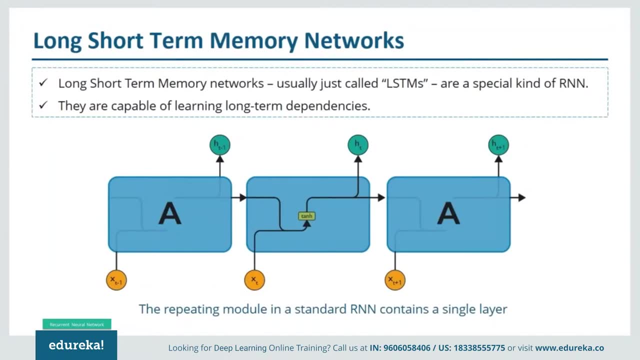 In this tutorial, we'll be discussing LSTMs, that are long short-term memory units. Now let us understand what exactly are LSTMs. So, guys, we saw what are the two limitations with the recurrent neural networks. Now we'll understand how we can solve that. 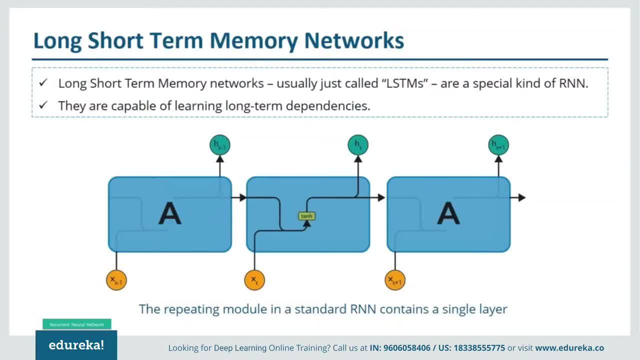 with the help of LSTMs. Now, what are LSTMs? Long short-term memory networks, usually called as LSTMs, are nothing but a special kind of recurrent neural network, And these recurrent neural networks are capable of learning long-term dependencies. 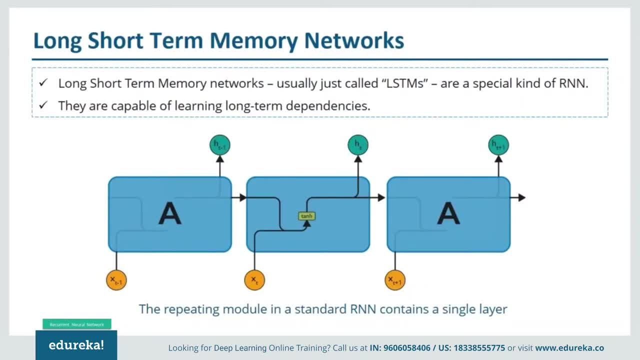 Now, what are long-term dependencies? I've discussed that in the previous slide, but I'll just explain it to you here as well. Now what happens? sometimes? we only need to look at the recent information to perform the present task. Now let me give you an example. 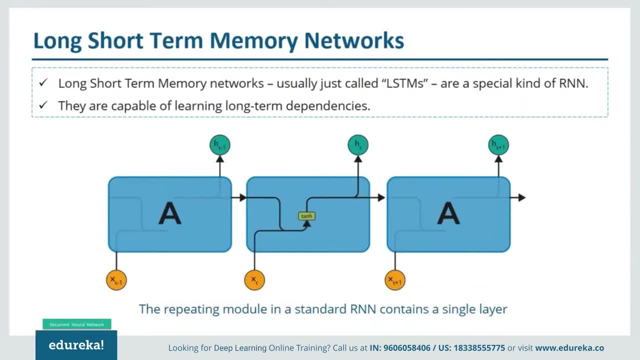 Consider a language model trying to predict the next word based on the previous ones. If we are trying to predict the last word in the sentence, say, the clouds are in the sky, So we don't need any further context. It's pretty obvious that the next word is going to be sky. 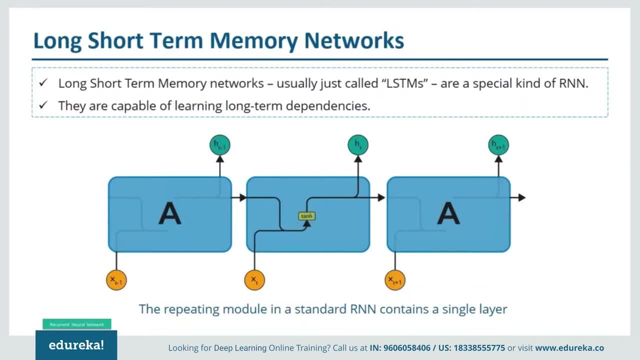 Now, in such cases where the gap between the relevant information and the place that it's needed is small, RNNs can learn to use the past information And at that time there won't be such problems like vanishing and exploring gradient. 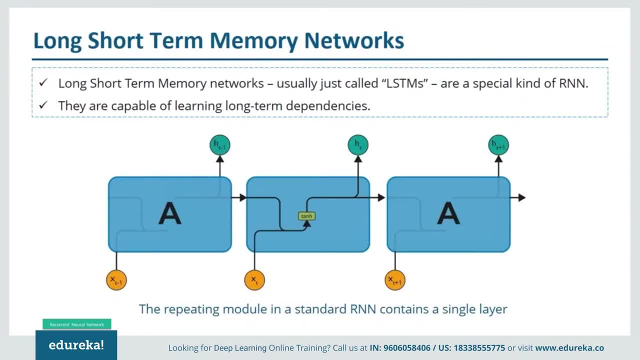 But there are a few cases where we need more context. Consider trying to predict the last word in the text. I grew up in France. Then there are some words After that comes. I speak fluent French. Now recent information suggests that the next word is probably the name of a language. 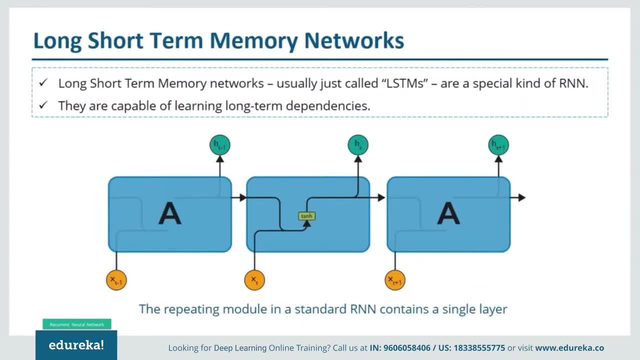 But if we want to narrow down which language, we need the context of France from further back, And it's entirely possible for the gap between the relevant information and the point where it is needed to become very large, And this is nothing but long-term dependencies. 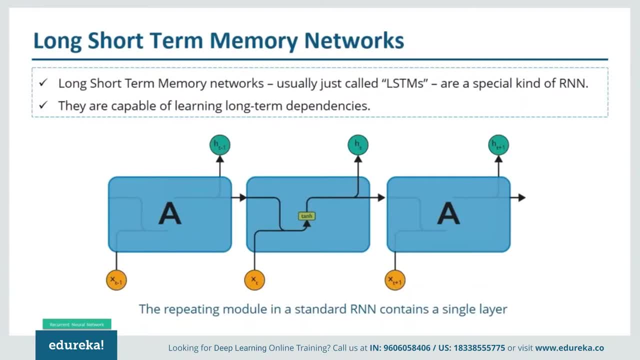 And the LSTMs are capable of handling such long-term dependencies. Now LSTMs also have a chain-like structure, like recurrent neural networks. Now all the recurrent neural networks have the form of a chain of repeating modules of neural networks Now in standard RNNs. 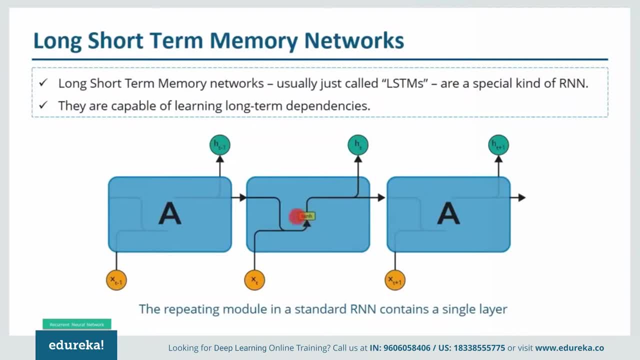 the repeating module will have a very simple structure, such as a single tanh layer that you can see Now. this tanh layer is nothing but a squashing function. Now, what I mean by squashing function is to convert my values between minus one and one. 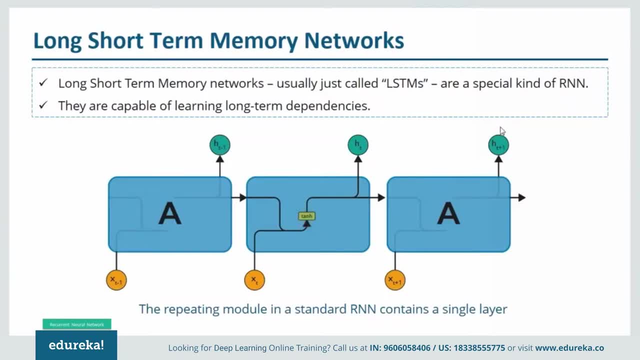 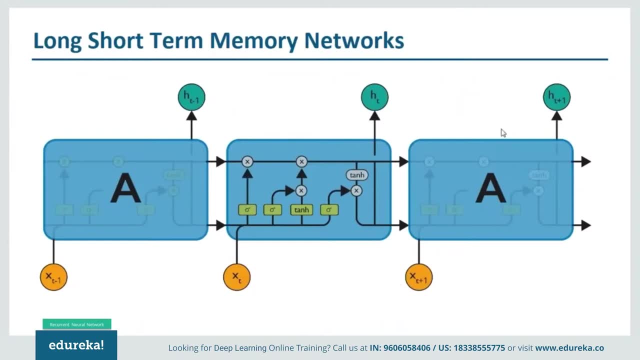 All right, that's why we use tanh, And this is an example of an RNN. Now we'll understand what exactly are LSTMs. Now this is a structure of an LSTM. If you notice, LSTM also have a chain-like structure. 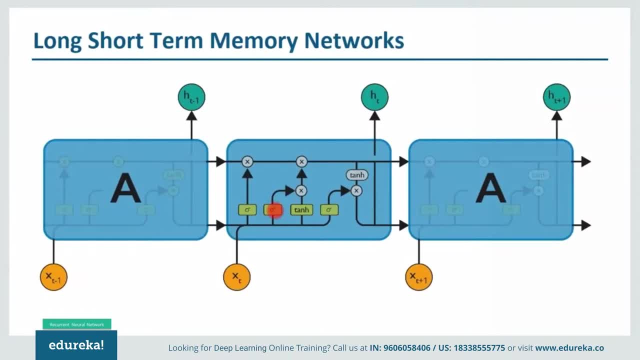 but the repeating module has different structures. Instead of having a single neural network layer, there are four, interacting in a very special way. Now, the key to LSTM is the cell state, Now this particular line that I'm highlighting, this is what is called the cell state. 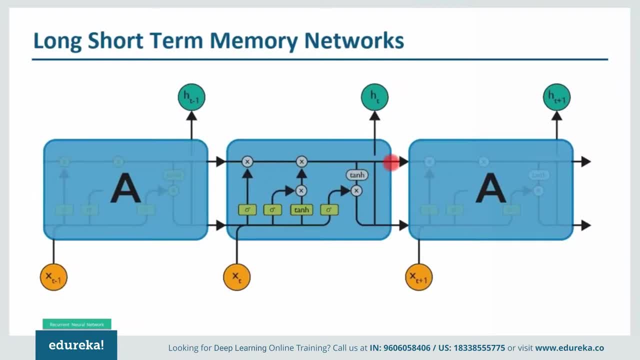 The horizontal line running through the top of the diagram. So this is nothing but your cell state. Now you can consider the cell state as a kind of a conveyor belt. It runs straight down the entire chain with only some minor linear interactions. Now, what I'll do? I'll give you a walkthrough. 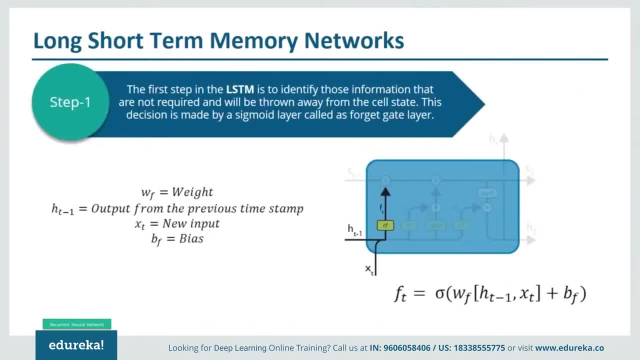 of LSTM step by step. all right, So we'll start with the first step. All right, guys. so the first step in our LSTM is to decide what information we are going to throw away from the cell state. And you know what is a cell state, right? 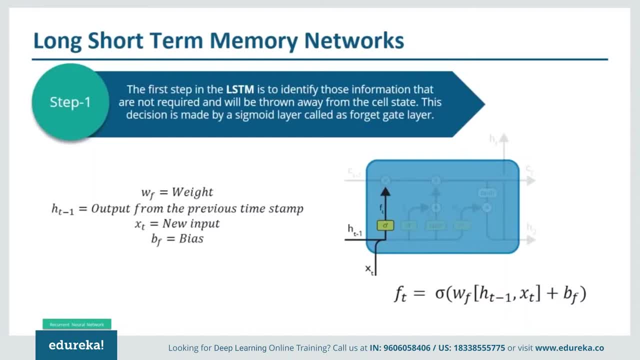 I've discussed in the previous slide. Now this decision is made by the same person, right? This decision is made by the sigmoid layer. So the layer that I'm highlighting with my cursor, it is a sigmoid layer called the forget gate layer. 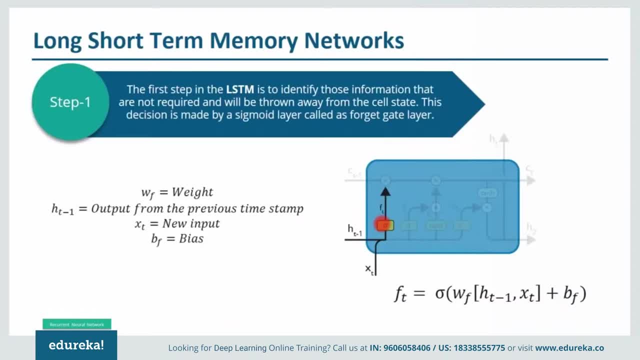 It looks at HT minus one, that is, the information from the previous time stamp, and XT, which is the new input, and outputs a number between zeros and one for each number in the cell state. CT minus one, which is coming from the previous time stamp. 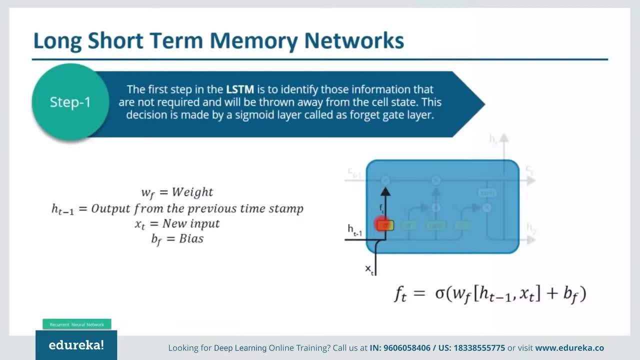 Our one represents completely keep this, while a zero represents completely get rid of this. Now, if we go back to our example of a language model trying to predict the next word based on all the previous ones, in such a problem, the cell state might include: 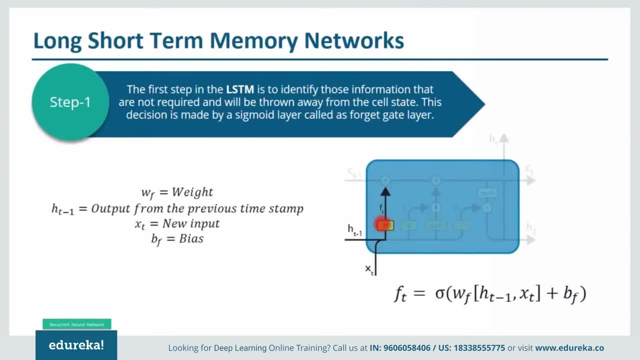 the gender of the present subject, so that the correct pronouns can be used When we see a new subject. we want to forget the gender of the old subject. right, We want to use the gender of the new subject, So we'll forget the gender of the previous subject here. 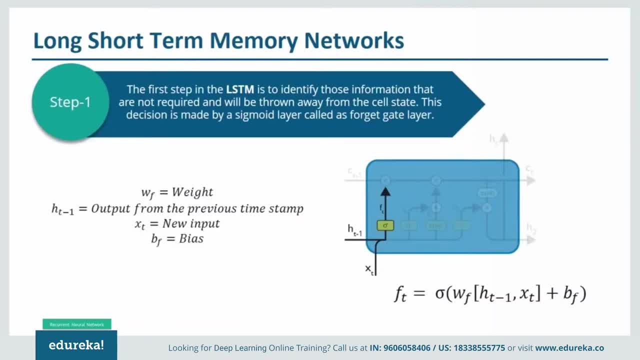 This is just an example to explain you what is happening here. Now let me explain you the equations which I've written here. So FT will be combining with the cell state. later on that I'll tell you. So, basically, FT will be nothing but the weight matrix. 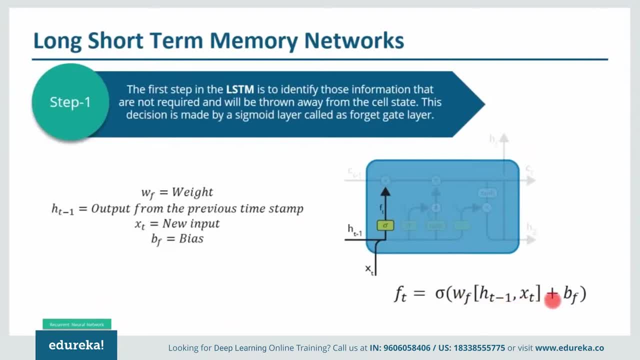 multiplied by HT minus one and XT and plus the bias, and this equation is passed through a sigmoid layer, all right, And we get an output that is zero and one. Zero means completely get rid of this and one means completely keep this, all right. 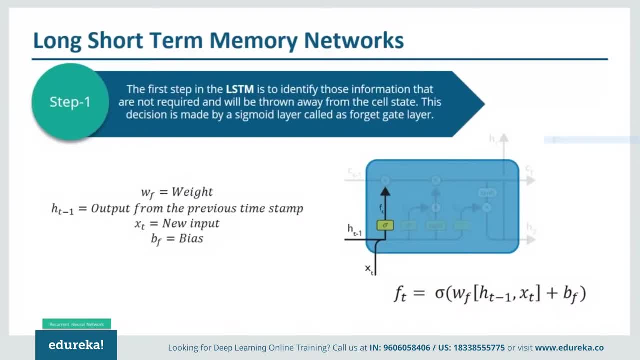 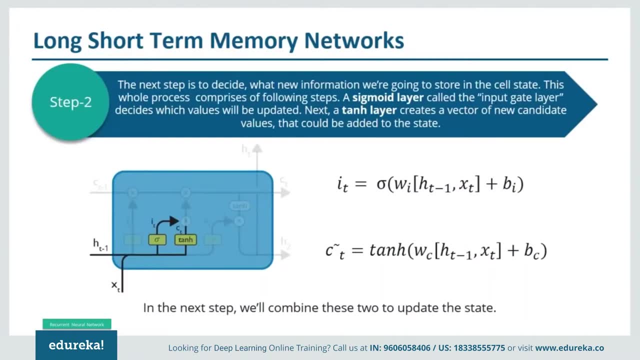 So this is what basically is happening in the first step. Now let us see what happens in the next step. So the next step is to decide what information we are going to store. In the previous step, we decided what information we are going to keep. 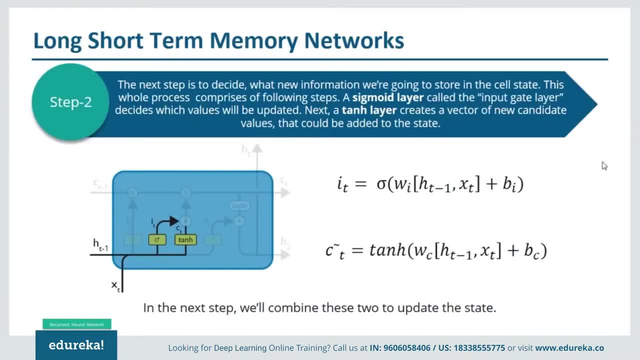 But here we are going to decide what information we are going to store here. all right, What new information we are going to store in the cell state. Now, this has two parts. First, a sigmoid layer. this is called a sigmoid layer. 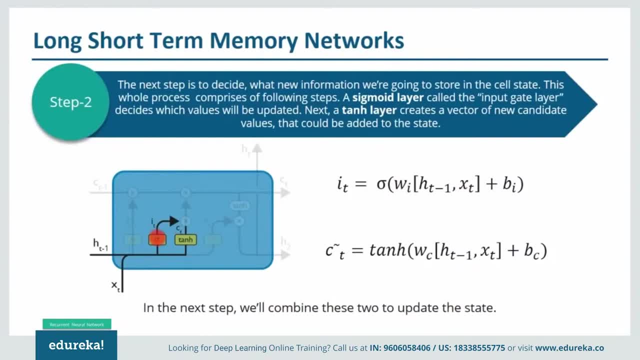 and which is also known as an input gate layer, decide which values we'll update. all right, So what values we need to update? And there's also a tanash layer that creates a vector of the candidate values. C bar of T minus one. 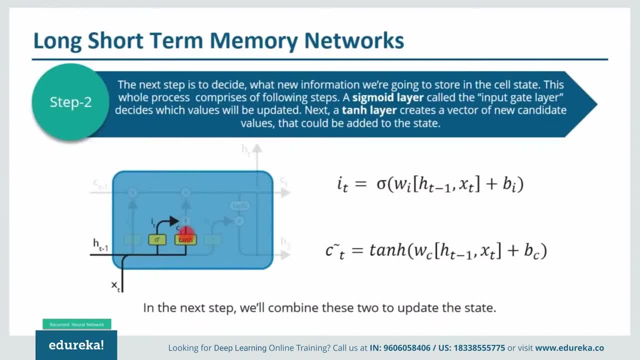 that will be added to the state later on. all right, So let me explain it to you in a simpler terms. So, whatever input that we are getting from the previous timestamp and the new input, it will be passed through a sigmoid function which will give us I of T. all right. 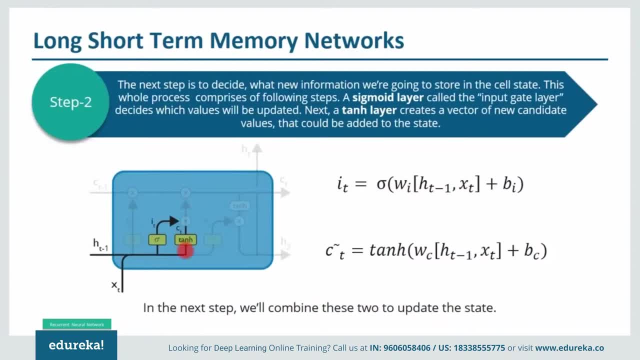 And this I of T will be multiplied by C T, which is nothing but the input coming from the previous timestamp and the new input but that is passed through a tanash. that will result in C T And this will be later added onto our cell state. 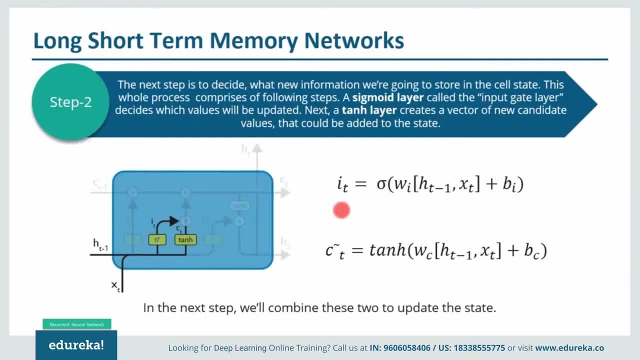 And the next step: we'll combine these two to update the states. Now let me explain the equations. So I of T will be what Weight matrix? and then we have H? T minus one comma, X T multiplied by the weight matrix plus the bias. pass it through a sigmoid function. 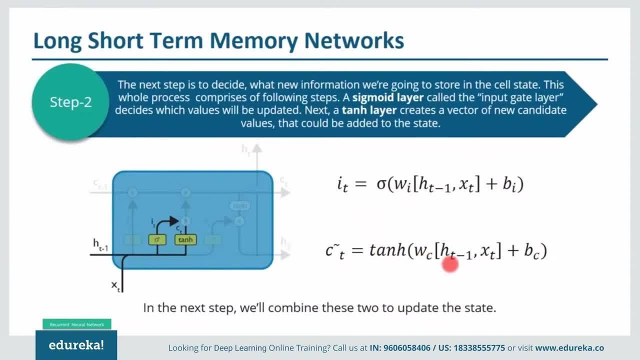 we get I of T, C bar of T, we'll get by passing a weight matrix- H T minus one, X T plus bias- through a tanash squashing function and we'll get C bar of T all right. So, as I've told you earlier as well, in the next step, 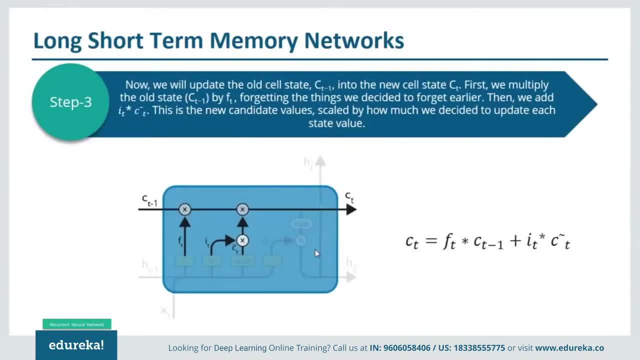 we'll combine these two to update the state. Let us see how we do that. So now is the time to update the old cell state C T minus one with the new cell state C T. all right, And the previous steps. we have already decided what to do. 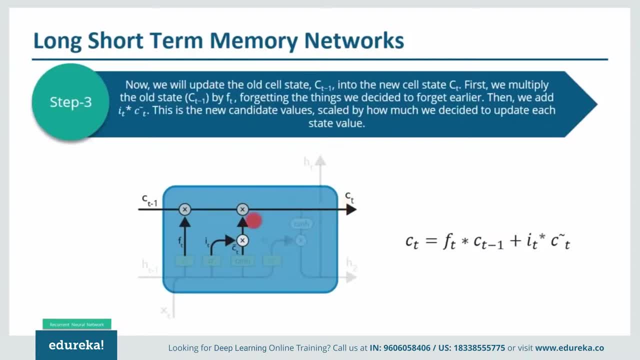 We just need to actually do it. So what we'll do? we'll multiply the old cell state C T minus one with F T that we got in the first step, forgetting the things that we decided to forget earlier in the first step, if you can recall, 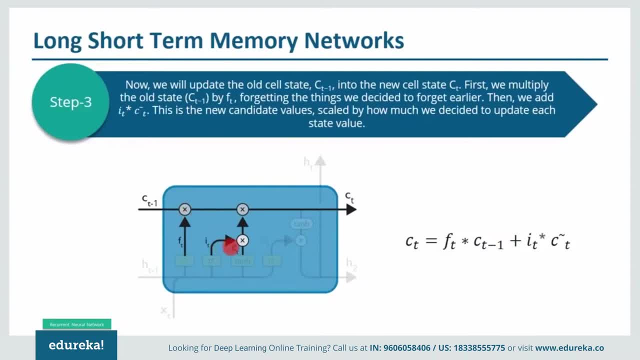 Then what we do? we add it to I T and C T, then we add it by the term that will come after multiplication of I T and C bar T, and this new candidate value is scaled by how much. we decided to update each state value. all right, 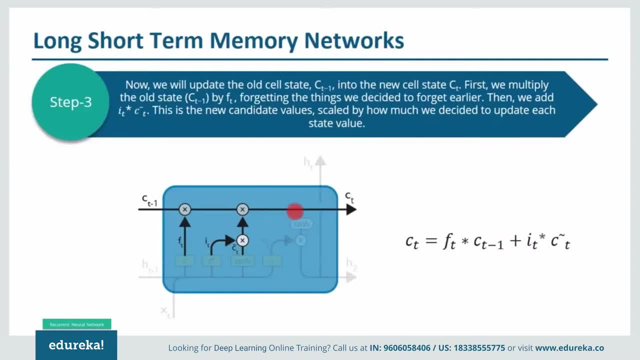 So in the case of the language model that we were discussing, this is where we would actually drop the information about the old subject- gender- and add the new information, as we decided in the previous steps. So I hope you are able to follow me, guys, all right? 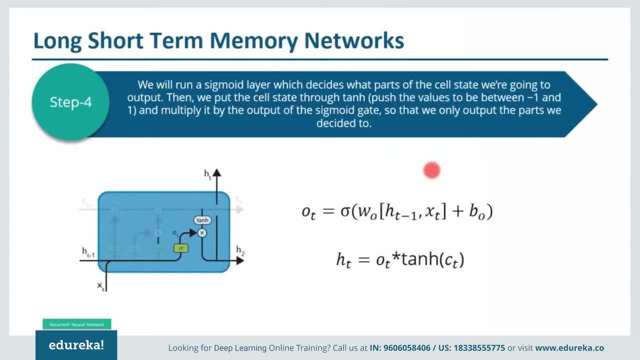 So let us move forward and we'll see what is the next step. Now, our last step is to decide what we are going to output, and this output will depend on our cell state, but it will be a filtered version. Now, finally, what we need to do is we need to decide. 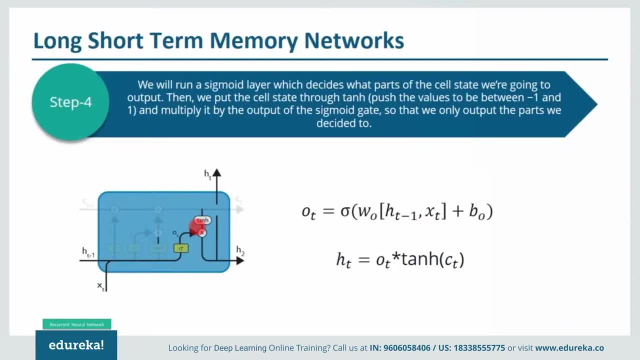 what we are going to output, and this output will be based on our cell state. First, we need to pass H- T minus one and X- three through a sigmoid activation function, so that we get an output that is O- T, all right. 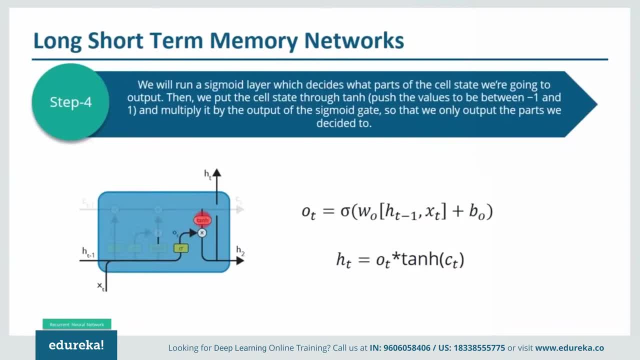 This O T will be in turn multiplied by the cell state after passing it through a tanh squashing function or an activation function. And why we do that? Just to push the values between minus one and one. So after multiplying O T, that is this value. 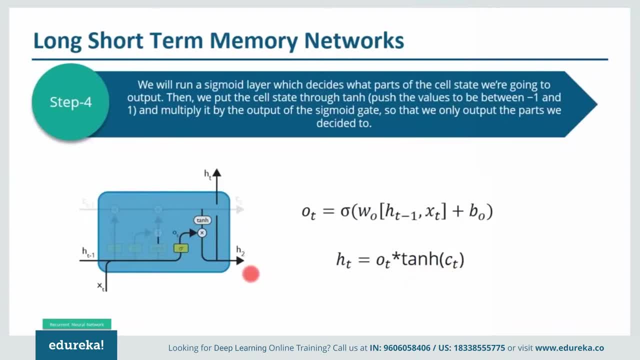 and a tanh C T, we'll get the output H two, which will be our new output, and that will only output the part that we decided to. Whatever we have decided in the previous steps, it will only output that value. all right, 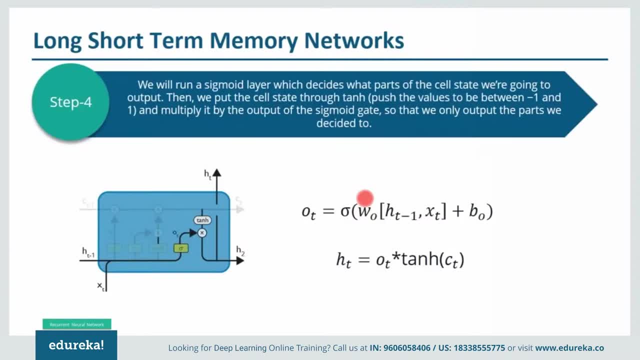 Now I'll take the example of the language model again. If I just saw a subject, it might want to output information relevant to a verb, and in case that's what is coming next, For example, it might output whether the subject is singular or plural. 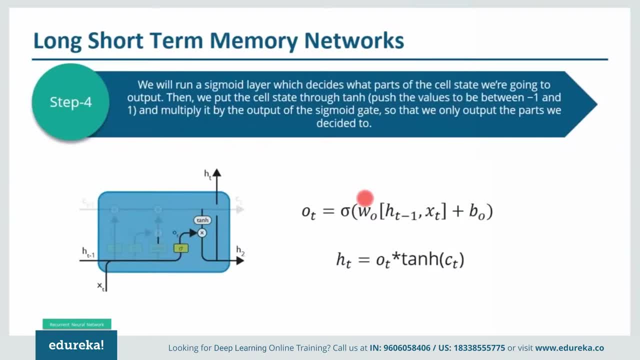 so that we know what form of a verb should be conjugated into. all right, And you can see from the. you can see the equations as well. Again, we have a sigmoid function, Then that whatever output we get from there, 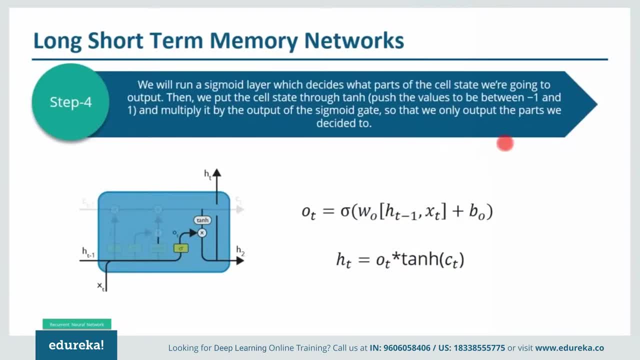 we multiply it with tanh, C, T to get the new output. All right, guys. so this is basically LSTMs and this is the LSTM function. So in the first step, we decided what we need to forget. In the next step, we decided what are we going to add? 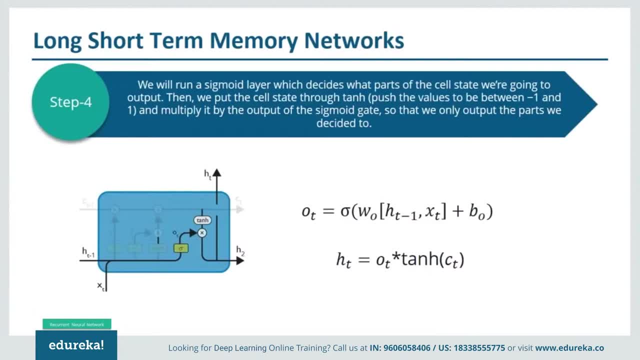 to our cell state, what new information we are going to add to our cell state, and we were taking an example of the gender throughout this whole process. all right, And in the third step, what we do. we actually combined it to get the new cell state. 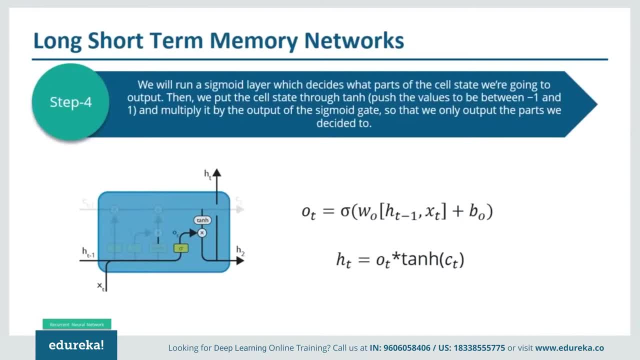 Now, in the fourth step, what we did. we finally got the output that we want. And how we did that? just by passing HT minus one and XT through a sigmoid function, multiplying it with the tanh C, T, and we get the new output. 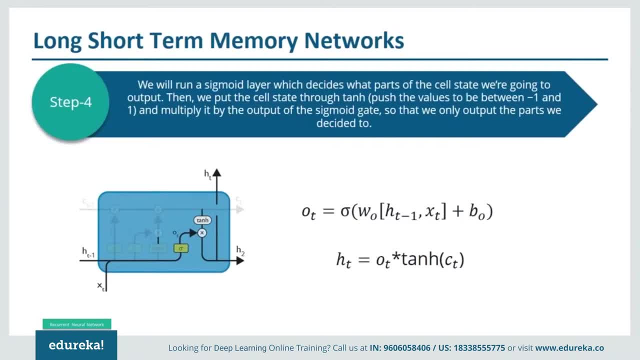 Fine, guys. So this is what basically LSTM is. guys, Now we'll look at a use case where we'll be using LSTM to predict the next word in a sentence. all right, Let me show you how we are going to do that. 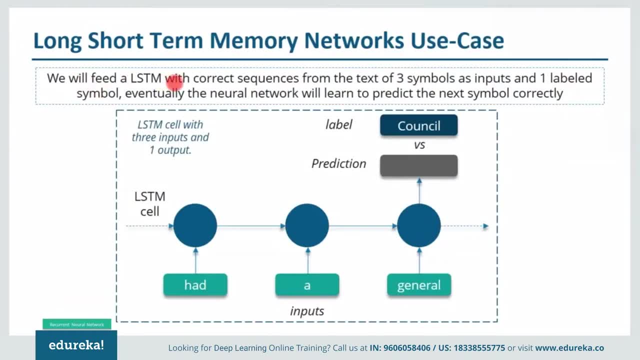 So this is what we are trying to do in our use case, guys. We'll feed our LSTM with correct sequences from the text of three symbols. For example, had a general and a label, that is, council in this particular example. Eventually, our network will learn. 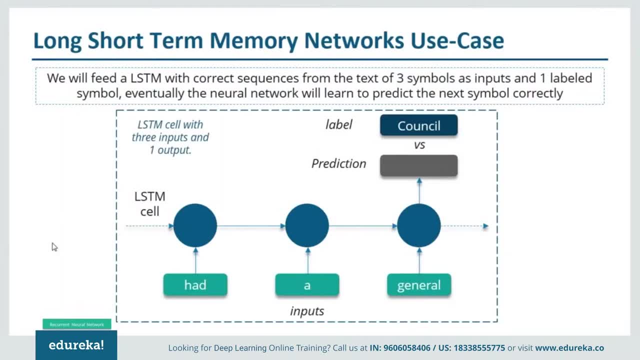 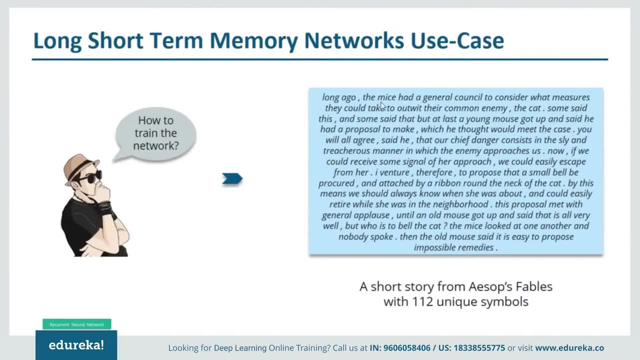 to predict the next symbol correctly, We need to train it on something. Let us see what we are going to train it on. So we'll be training our LSTM to predict the next word using a sample short story that you can see over here. 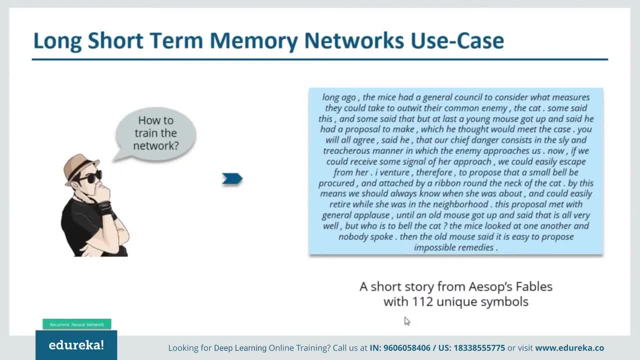 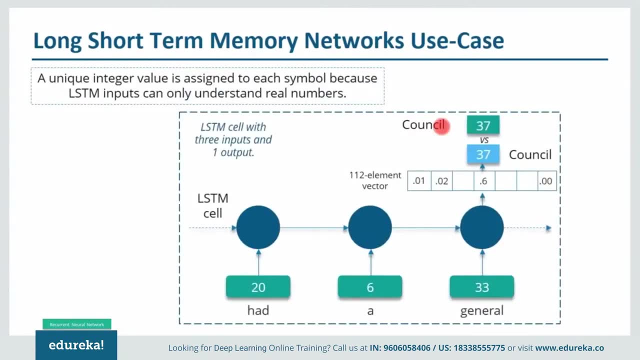 All right, so it has basically 112 unique symbols, So even comma and full stop are considered as symbols. All right, so this is what we are going to train it on. So, technically, we know that LSTMs can only understand real numbers. all right. 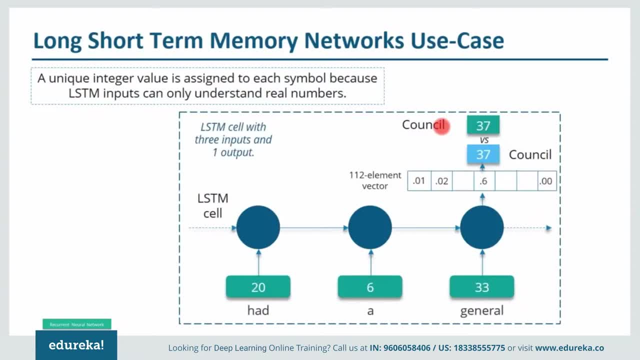 So what we need to do is we need to convert these unique symbols into a unique integer value based on the frequency of occurrence, And like that, we'll create a dictionary. For example, we have had here that will have value 20.. A will have value six. general will have value 33.. 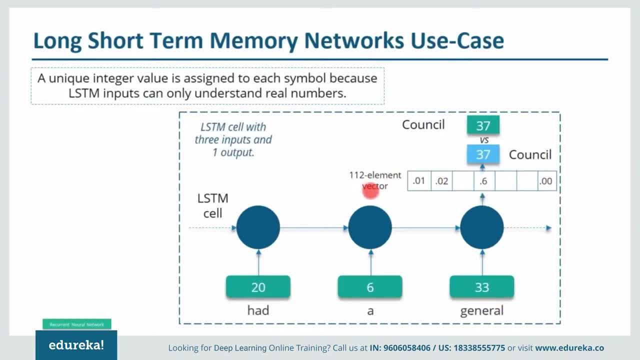 All right, and then what happens? our LSTM will create 112 element vector that will contain the probability of each of these words or each of these unique integer values. all right, So, since 0.6 has the highest probability in this particular vector, 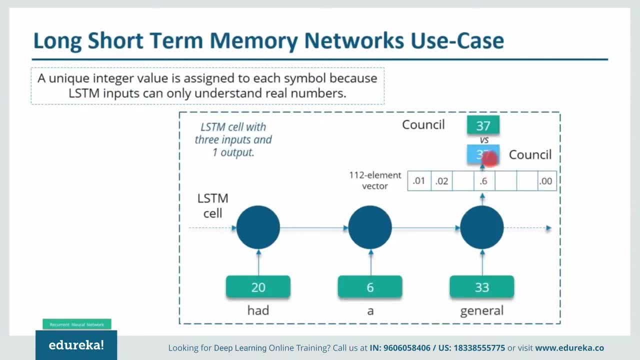 it'll pick the index value of 0.6.. Then it will see what symbol is attached to that particular particular integer value. So 37 is attached to council. So this will be our prediction, which is absolutely correct, as a label is also council, according to our training data. 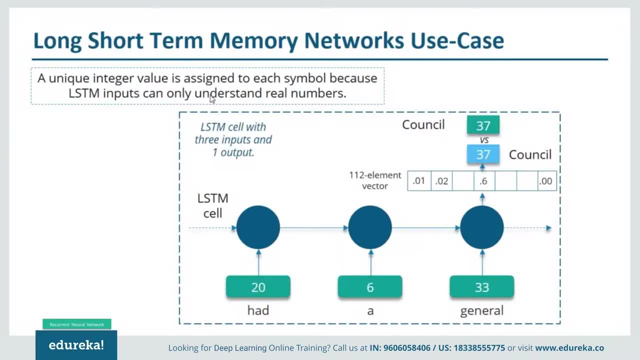 All right, so this is what we are going to do in our use case. So, guys, this is what we'll be doing in today's use case. Now I'll quickly open my PyCharm and I'll show you how you can implement it using Python. 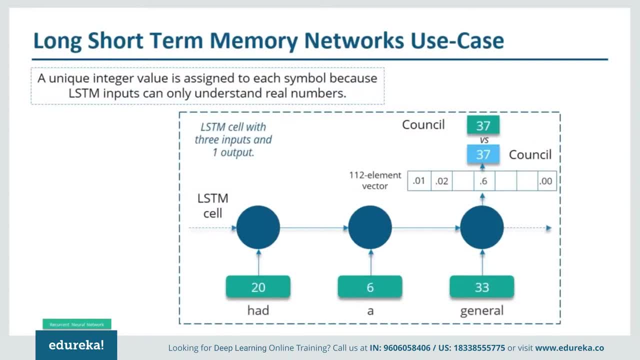 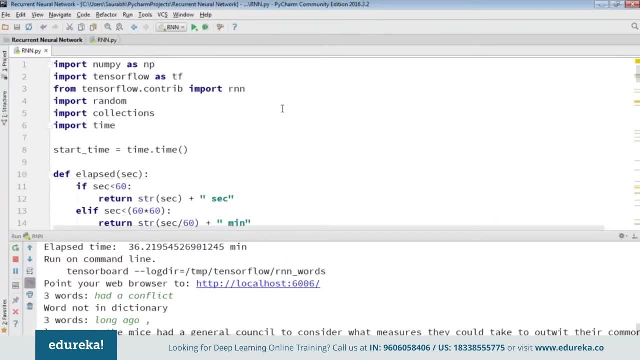 We'll be using TensorFlow, which is a popular Python library for implementing deep neural networks or neural networks in general. All right, so I'll quickly open my PyCharm now. So, guys, this is my PyCharm, and over here I've already written the code. 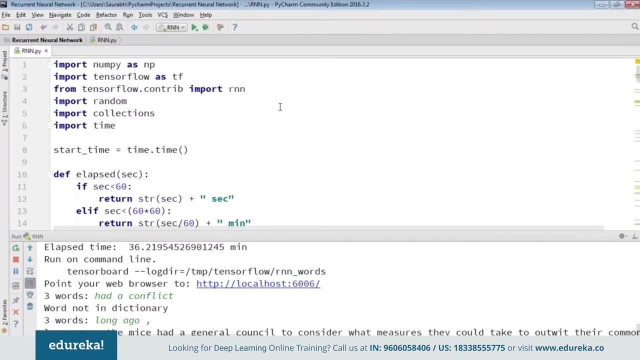 in order to execute the use case that we have. So first we need to do is import the libraries NumPy, Ferraris, TensorFlow- we know TensorFlowcontra. From that we need to import RNN in random collections in time. 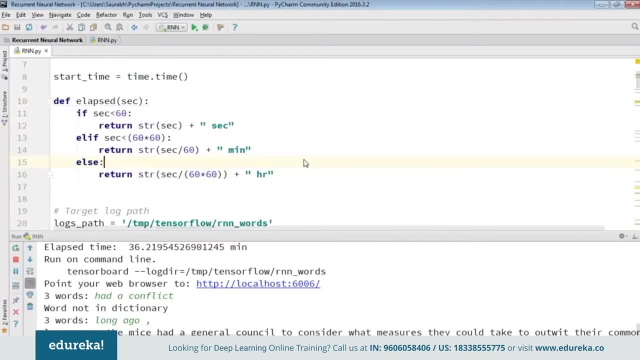 All right, so this particular block of code is used to evaluate the time taken for the training. After that, we have log underscore path, and this log underscore path is basically telling us the path where the graph will be stored. All right, so there'll be a graph that will be created. 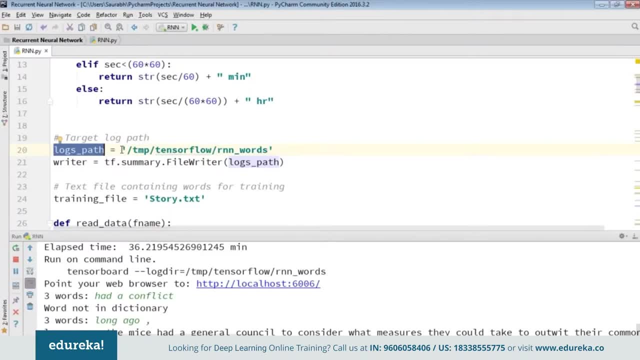 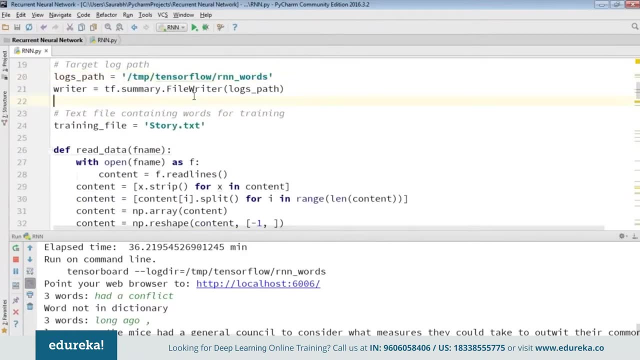 and then that graph will be launched, Then only our RNN model will be executed. Then that's how TensorFlow works, guys, So that graph will be created in this particular path. All right, and we are using summary writer, So that'll actually create the log file. 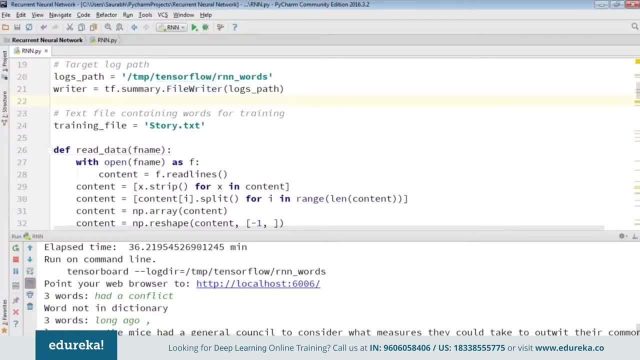 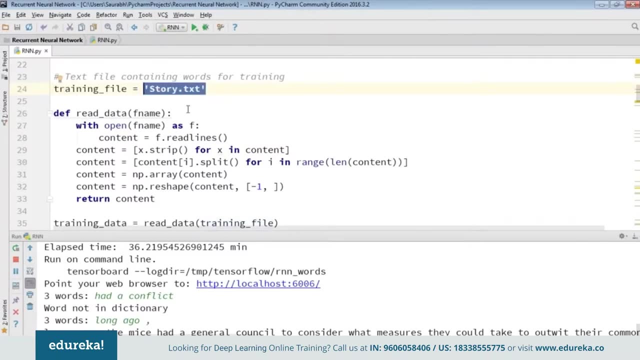 that will be used in order to display the graph using TensorFlow. All right, so then we have defined training underscore file, which will have our story, on which we'll train our model on. Then what we need to do is read this file. So how are we gonna do that? 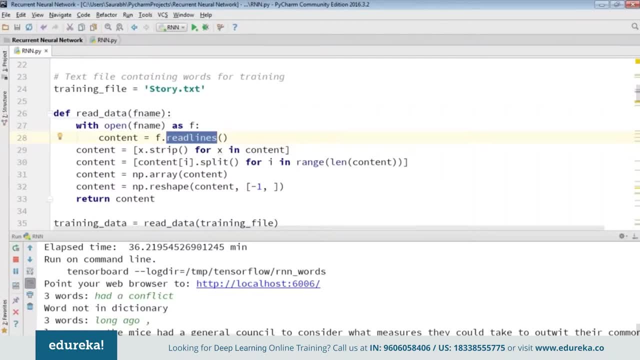 First is read line by line whatever content that we have in our file. Then we are going to strip it. that means we are going to remove the first and the last white space. Then again we are splitting it just to remove all the white spaces that are there. 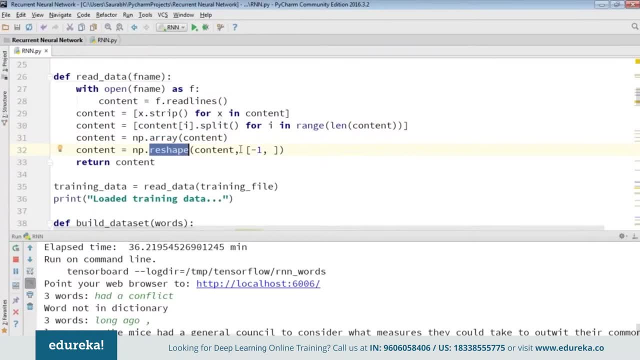 After that, we're creating an array and then we are reshaping it. Now, during the reshape, if you notice this minus one value tells us the compatibility. All right. so when you're reshaping it, you need to make sure that you know. 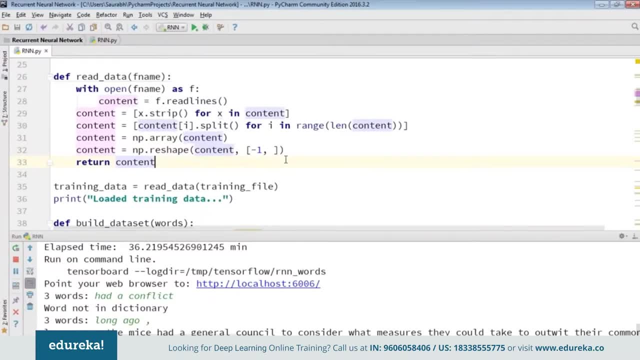 we are providing the correct parameters to reshape it, So you can convert a three cross two matrix to a two cross three matrix, right? So just to make sure that it is compatible enough, we add this minus one And it'll be done automatically. all right. 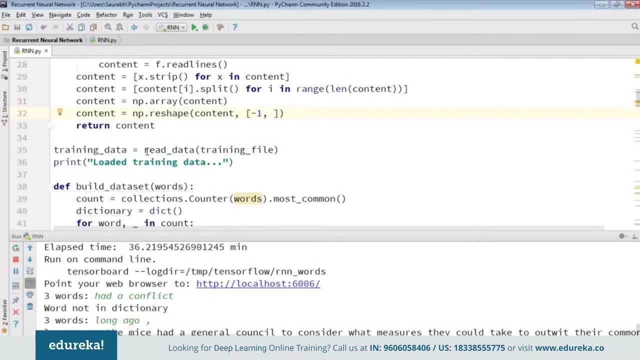 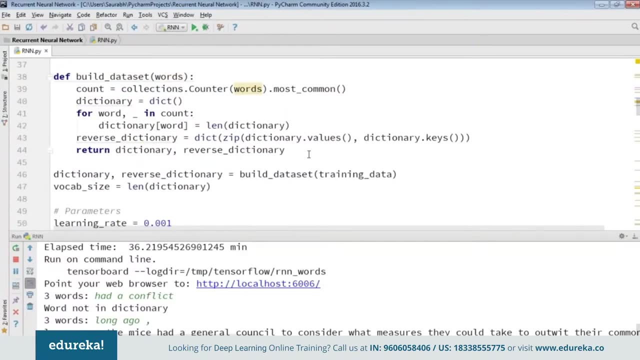 Then return content. After that, what we are doing, we are feeding in the training data that we have training underscore file. We are feeding in our story and calling the function: read underscore data. Then what we are doing, we are creating a dictionary. 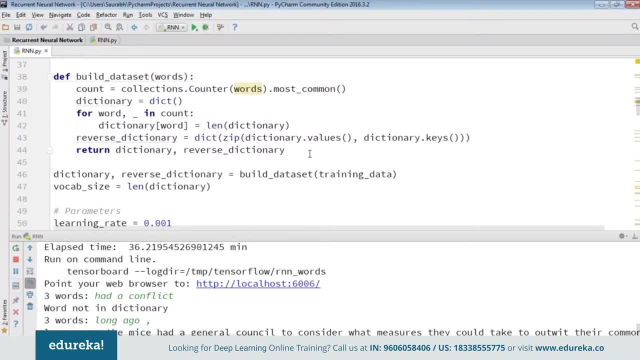 What is a dictionary? We all know key value pairs based on the frequency of occurrences of each symbol. All right, so from here, collections, dot, counter words, dot, most common, So most common words with their frequency of occurrence, there'll be a dictionary created. 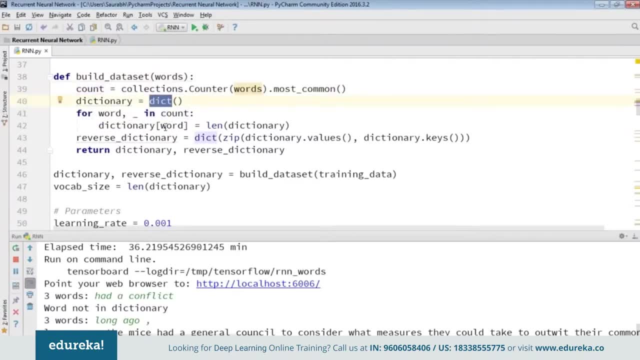 And after that we'll call this dict function, and this dict function will feed in word, and which is equal to length of dictionary. That means whatever the length of that particular dictionary is how many time it is repeated. So we'll have the frequency as well as the symbol. 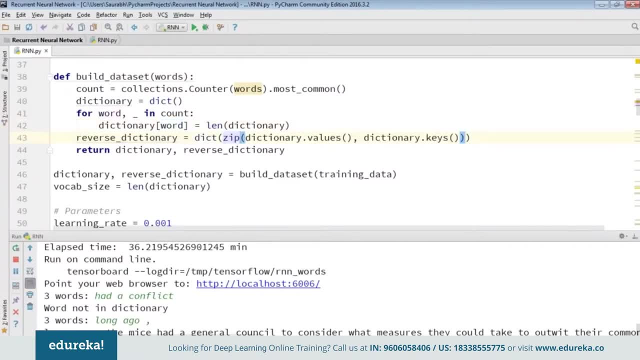 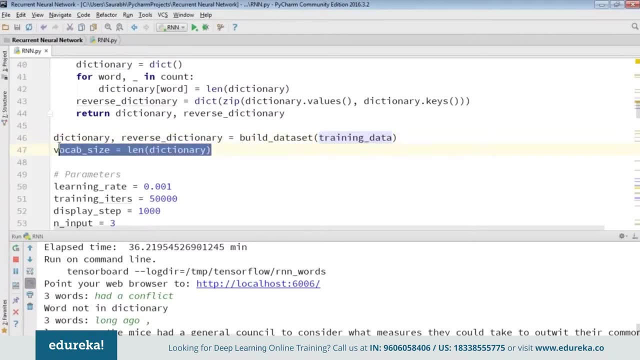 That'll be our key value pair, and we are reversing it as well. Then what we are doing? we are calling it build underscore data set and we're feeding in our training data there. This is our vocabulary size, which is nothing but the length of your dictionary. 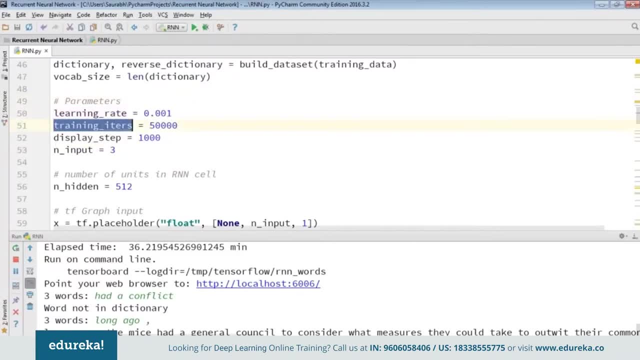 Then we have defined various parameters, such as learning rate, iterations or epochs. Then we have display, step and underscore input. Now, learning rate? we all know what it is, The steps in which our variables are updated. Training, underscore, iterations is nothing but your epochs. 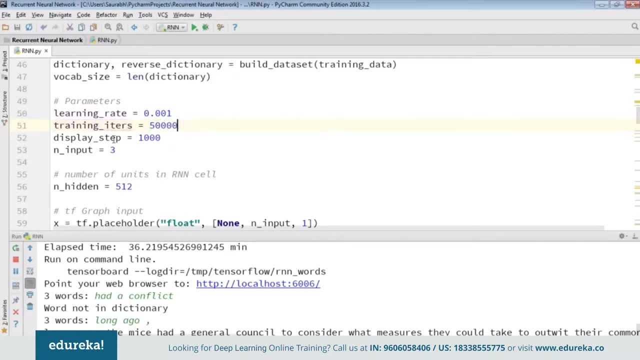 the total number of iterations. So we have given 50,000 iterations here. Then we have display underscore step. that is thousand, which is basically your batch size. So batch size is what? After every thousand epochs, you'll see the output. 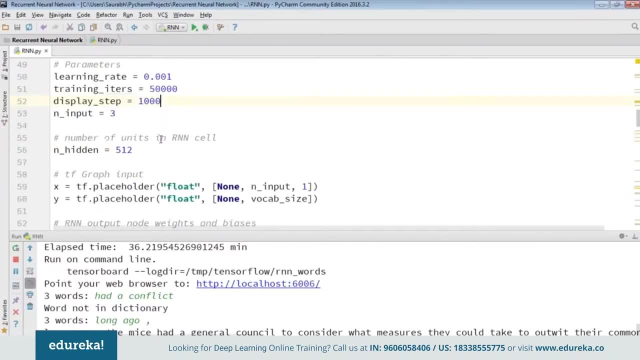 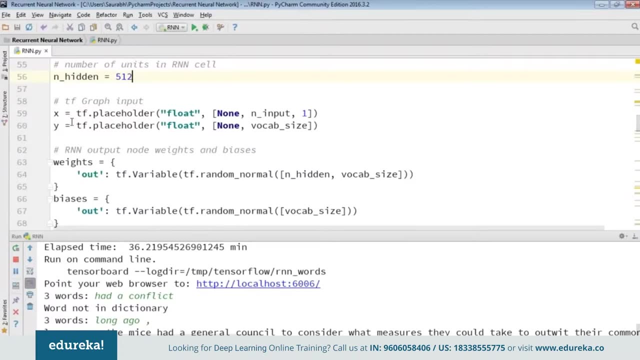 All right, so it'll be processing it in batches of thousand iterations. Then we have n underscore input as three. Now the number of units in the RNN cell will keep it as 512.. Then we need to define x and y, So x will be our placeholder. 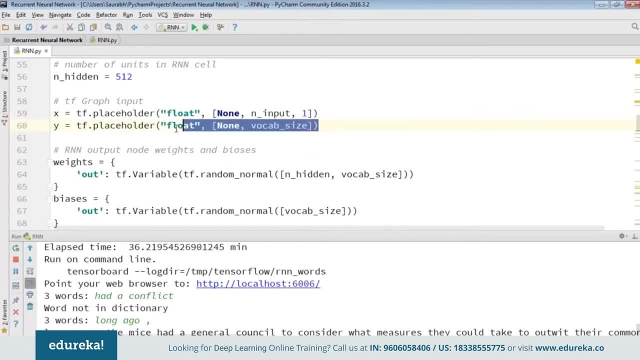 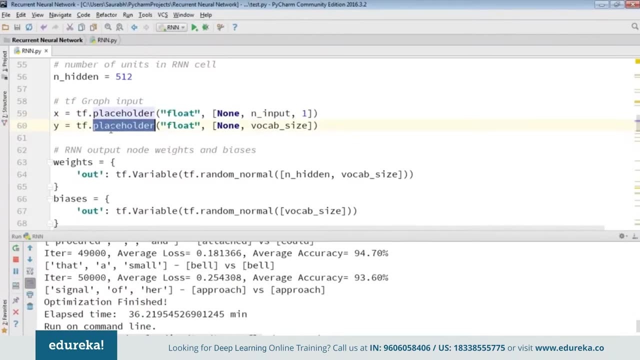 that will have the input values and y will have all the labels, all right. Vocab size. So x is a placeholder where we'll be feeding in our input dictionary. Similarly, y is also one word placeholder and it'll have a shape of none comma. vocab size. 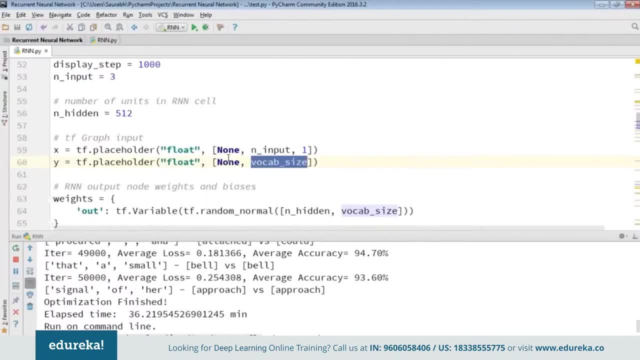 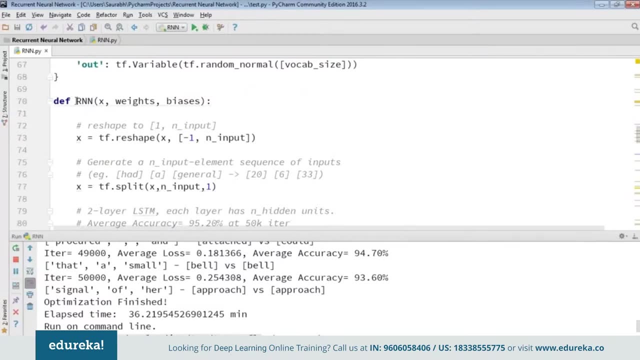 Vocab size we have defined earlier, as you can see, which is nothing but the length of your dictionary. Then we are defining weights as well as biases. After that, we have defined our model, all right, So this is how we are going to define it. 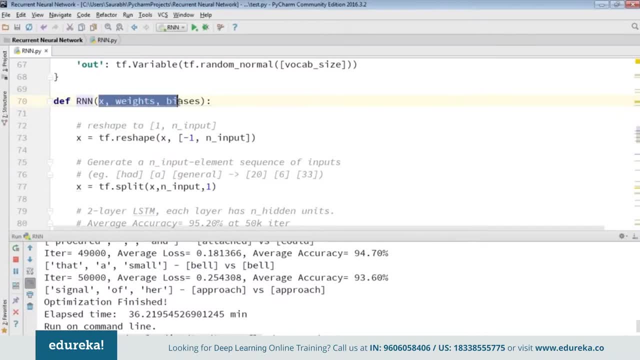 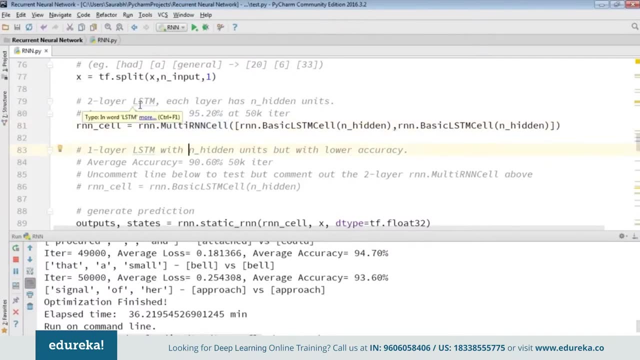 we'll create a function RNN, when we'll have x weights and biases, And after that we are calling in RNN, dot, multi RNN cell function. And this is basically to create a two-layer LSTM and each layer has n underscore- hidden units. 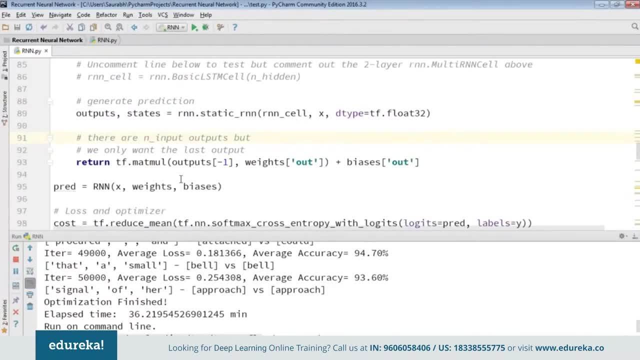 After that, what we are doing? we are generating the predictions. But once we have generated the prediction, there are n underscore input outputs, but we only want the last output, all right, So for that we have written this particular line. 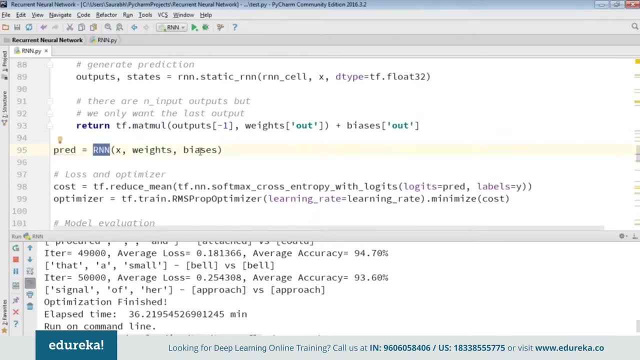 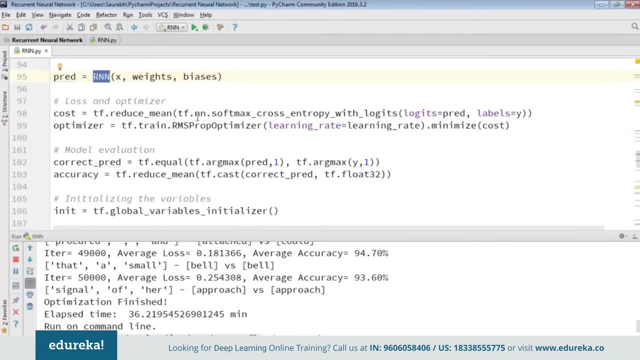 And then, finally, we are making a prediction. we are calling this RNN function, feeding in x weights and biases. After that we are calculating the loss and then we are optimizing it. For calculating the loss, we are using: reduce, underscore, mean, softmax, cross entropy. 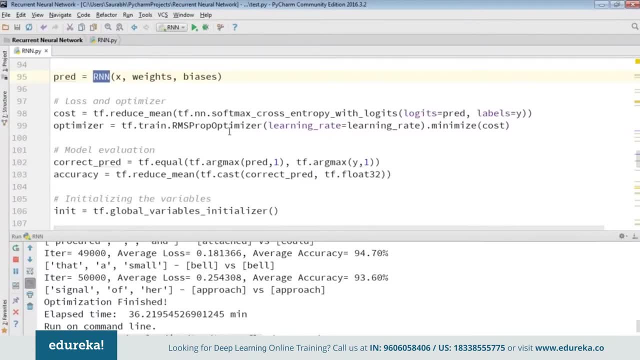 and this will give us basically the probability of each symbol. and then we are optimizing it using RMS prop optimizer. all right, And this gives actually a better accuracy than Adam optimizer, and that's the reason why we are using it. Then we are going to calculate the accuracy. 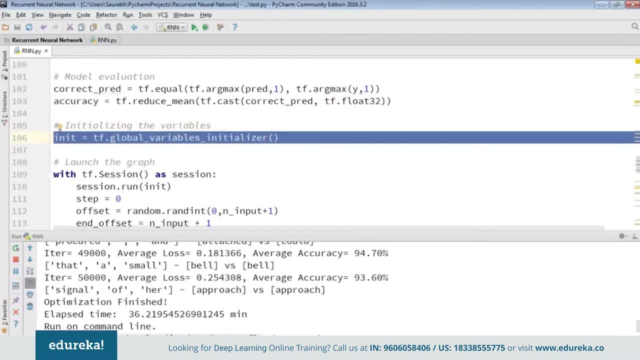 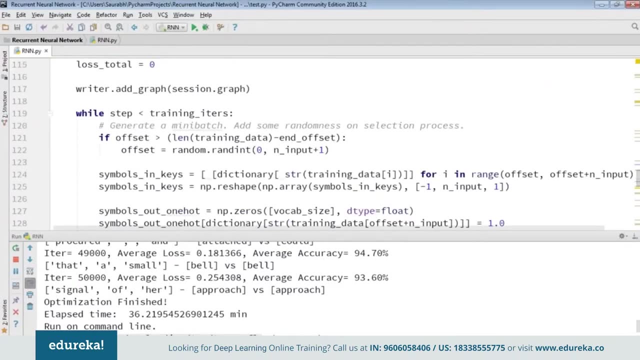 and after that we are going to initialize the variables that we have used, As we have seen in TensorFlow that we need to initialize all the variables, unlike constants and placeholders in TensorFlow, all right, And once we are done with that, we are feeding in our values. 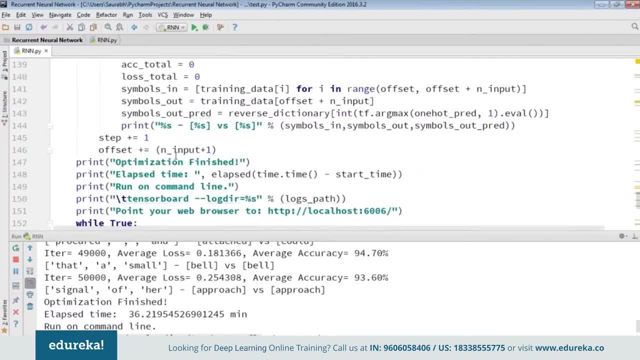 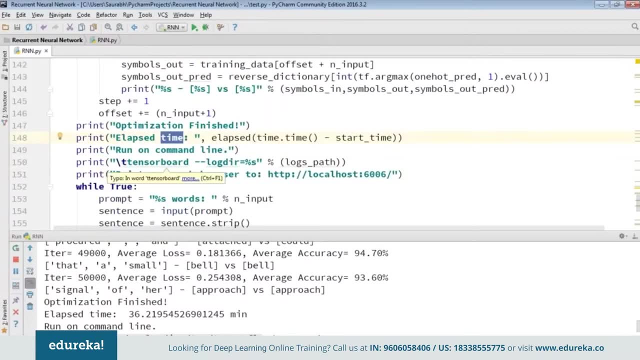 then calculating the accuracy, how accurate it is, and then, when optimization is done, we are calculating the elapsed time as well, so that will give us how much time it took in order to train our model. Then this is just to run the TensorBoard. 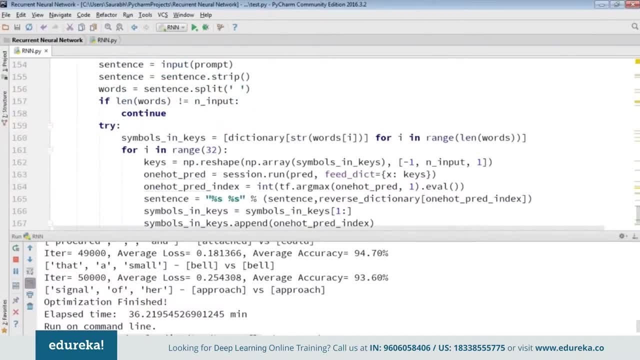 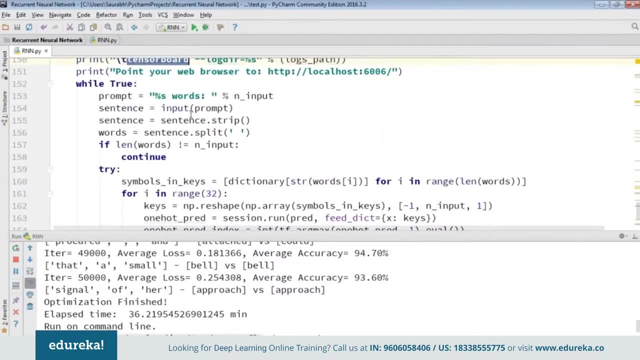 on localhost 6006,. and yeah, and this particular block of code is used in order to handle the exceptions, So exceptions can be like: whatever word that we are putting in might not be there in our dictionary or might not be there in our training data. 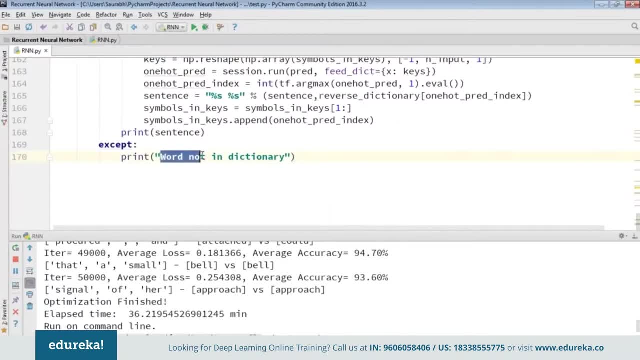 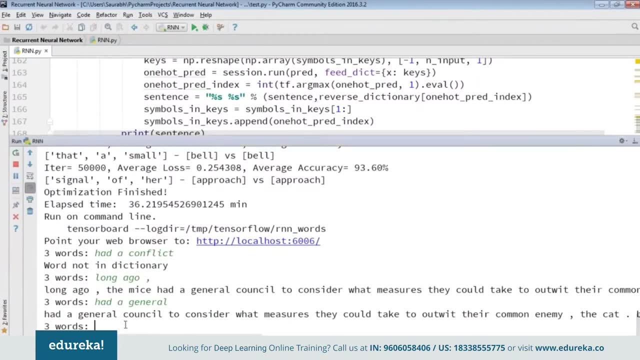 So those exceptions will be handled here, and if it is not there in our dictionary, then it'll print word not in our dictionary, All right. so fine guys, let's input some values and we'll have some fun with this model, all right? 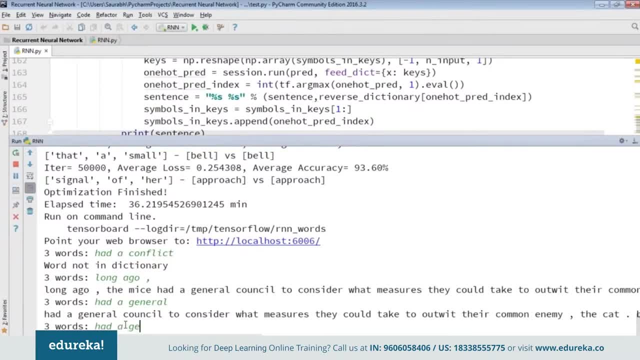 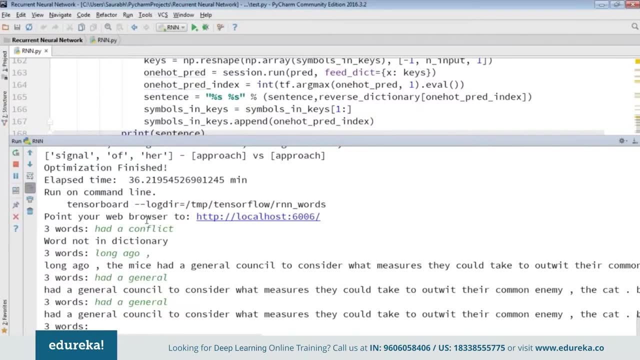 So the first thing that I'm gonna feed in is had a general. So whenever I feed in these three values had a general, there'll be a story that will be generated by feeding back the predicted output as the next symbol in the inputs. all right, 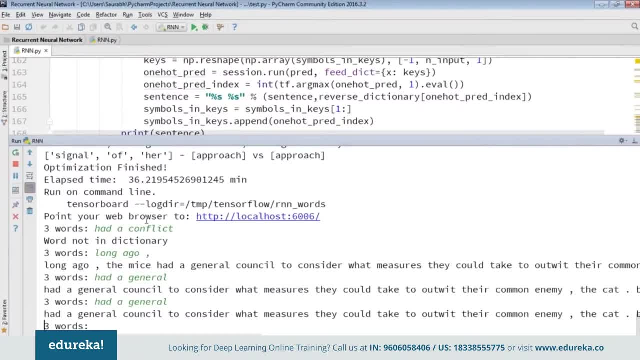 So when I feed in, had a general, so it'll predict the correct output as council and this council will be fed back as a part of the new input and our new input will be a general council, so it'll be a general council, all right. 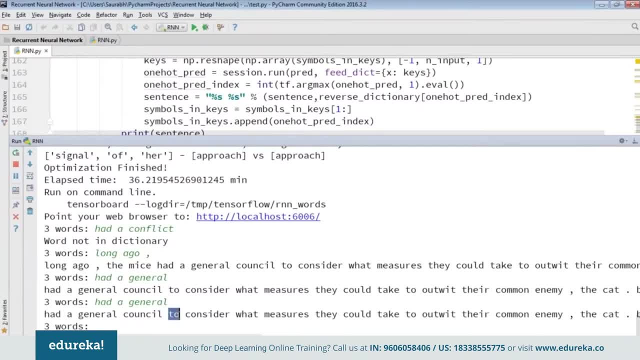 So these three words will become our new input to predict the new output, which is two all right, and so on. So, surprisingly, LSTM actually creates a story that somehow makes sense. so let's just read. it Had a general council to consider what measures. 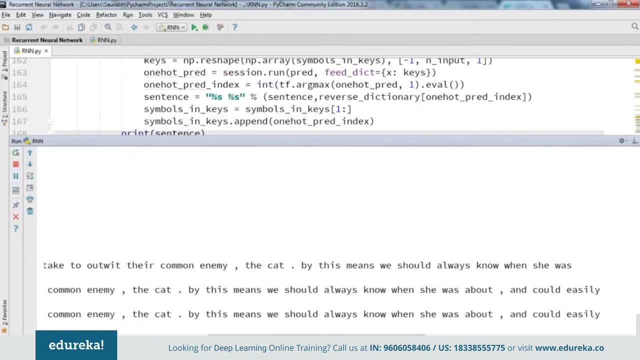 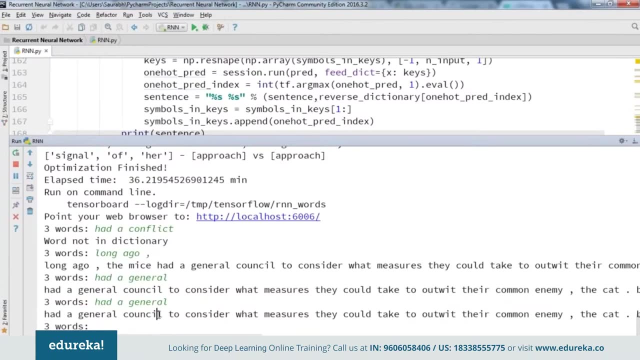 they could take to outwit their common enemy, the cat. This means we should always know when she was about and could easily all right, So somehow it actually makes sense when you feed in that. So what'll happen when you feed in these three inputs? 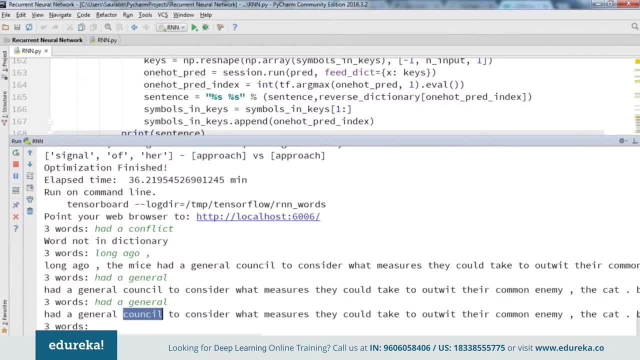 it'll predict the next word, that is, council. After that it'll take council and it'll feed back as an input along with a general. So a general council will be your next input to predict two Similarly in the next iteration. 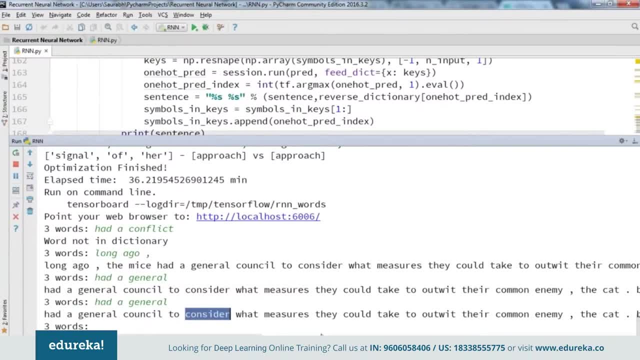 it'll take general council two and predict, consider for us, and this will keep on repeating. So, guys, this is it for today's session. Now let me just give you a quick summary of what all things we have discussed. So, guys, we started by understanding. 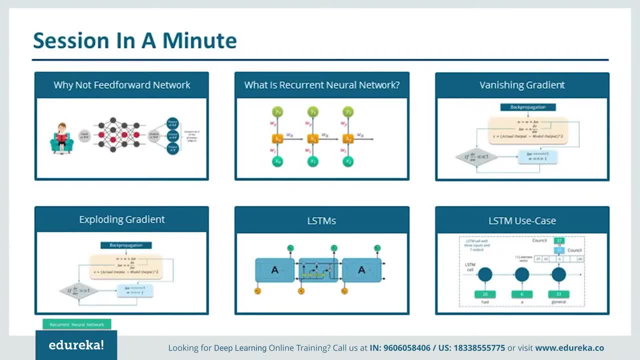 why can't we use feed-forward networks? for various problems We understood few limitations of feed-forward networks. Then we saw how recurrent neural networks solves those problems and what exactly it is. After that we saw various issues with recurrent neural network as well. 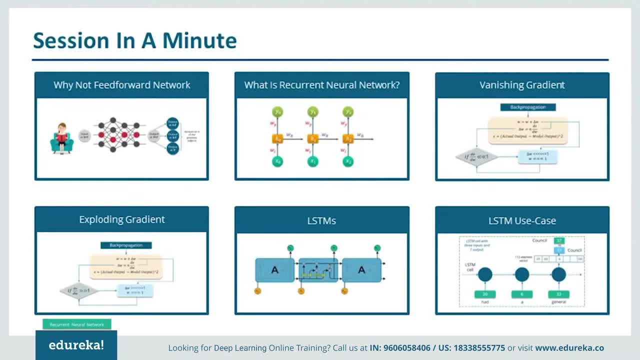 vanishing and exploring gradient, and both of these issues are due to long-term dependencies. Now, in order to solve those issues because of long-term dependencies, we use long short-term memory networks called LSTMs. So we understood what exactly LSTM is. 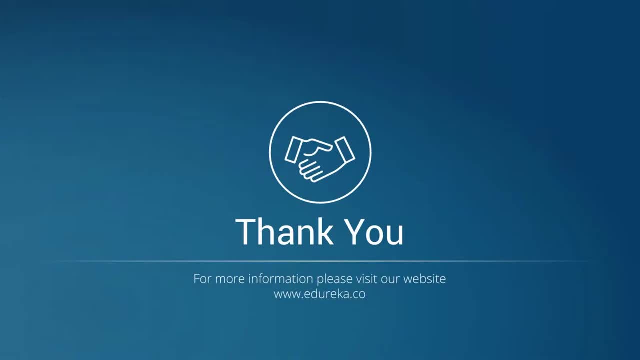 and after that we even saw use case of LSTM. So, guys, this is it for today's session. Thank you and have a great day. Thank you.